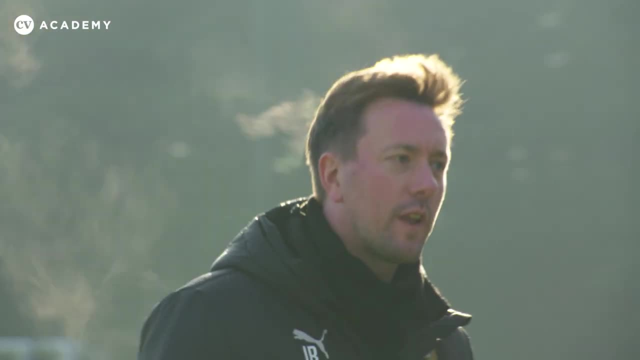 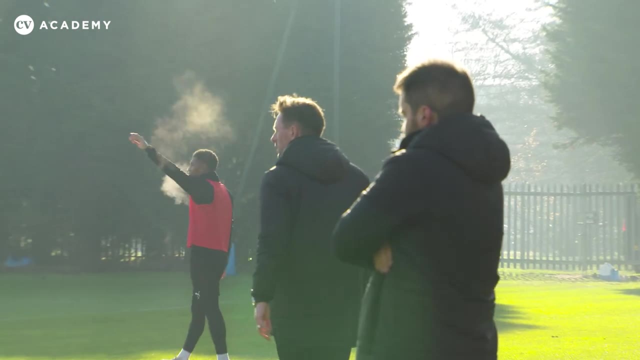 Look for certain key things in that training, clip them, send them to the players, just to give continual feedback to the players so that it doesn't just stop when training finishes but it carries on after that. As Gaffer said, it's important to know what he's looking at. 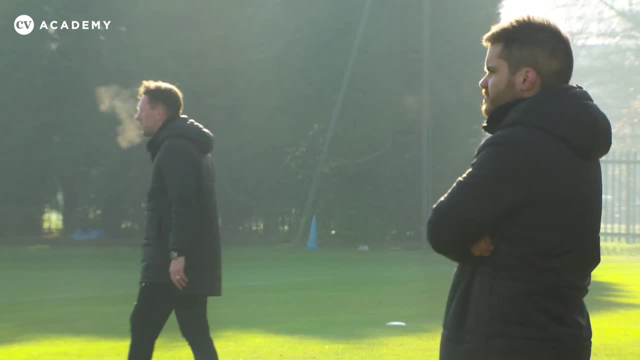 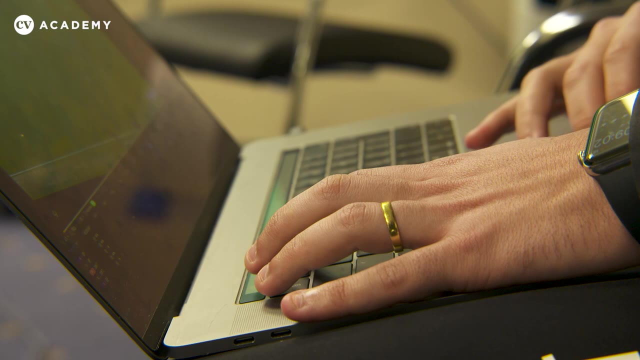 And if I don't have that, it's very, very hard to actually show him what he wants. But the goal is to look at the game kind of through his eyes a little bit. That's why the connection is important and why it's important to know exactly what we're after. 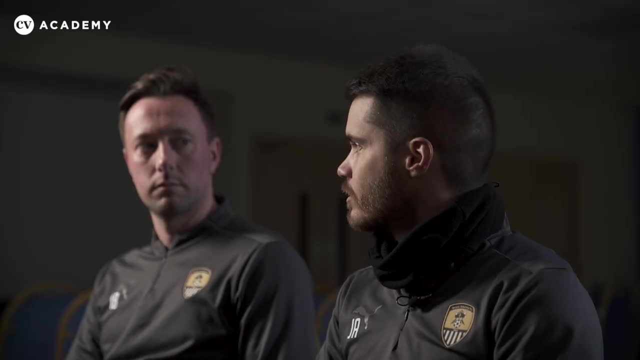 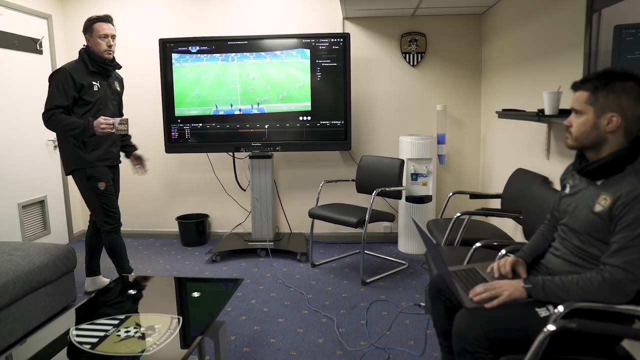 Then I can just go and look for it and take a bit of load off of Gaffer's plate and deliver it to the players a bit. We're always in touch. We're always quite clear on what we're after and what's good behaviour. 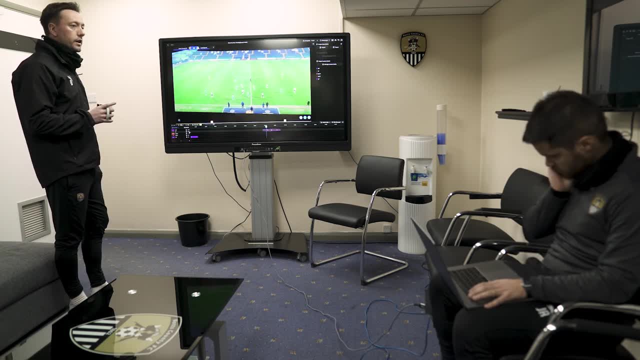 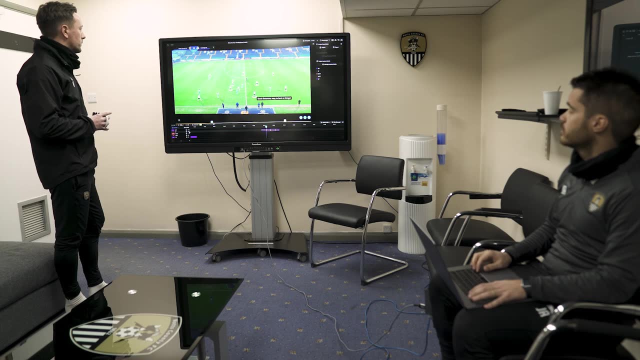 what's behaviour that we want to improve. So I would just say it's a good, healthy relationship with a lot of clarity For me to do my job- very important- And for Ian to get the best out of me for sure as well. 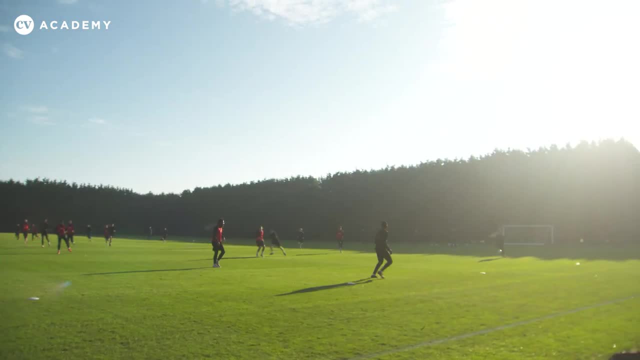 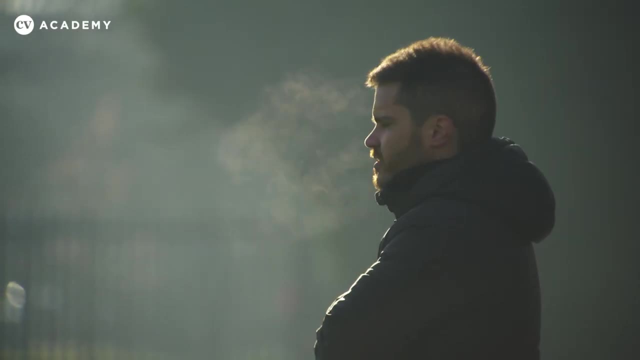 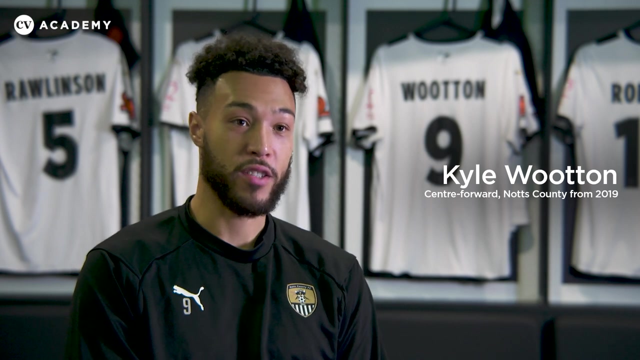 Go on, go on, go on. Yeah, I've got him. If you can watch things as a team and as an individual with certain coaches and things that you're working on, it's a massive advantage. I mean Zhao- I've just been speaking with him there. 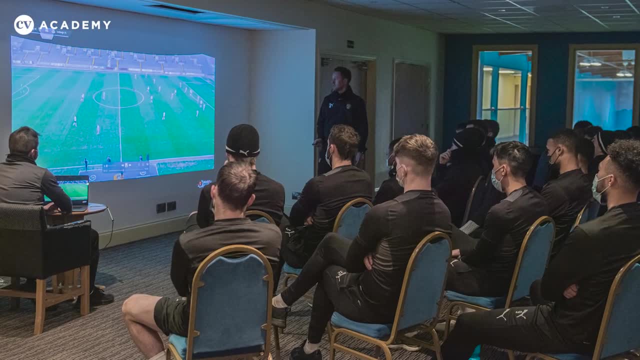 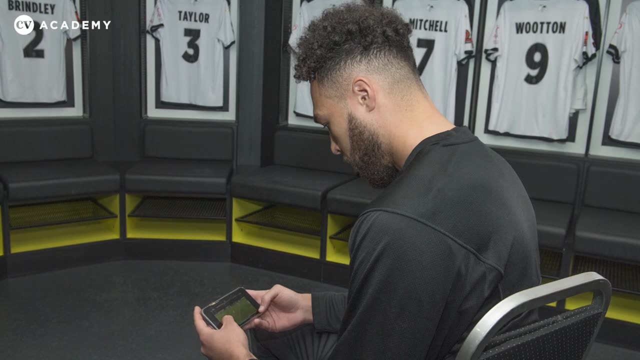 and he always sends me clips of certain strikers who are sort of similar or want that sort of movement and things, And the Gaffers sent me videos as well on the B Pro. I think he's got a good relationship with certain strikers, what he wants. 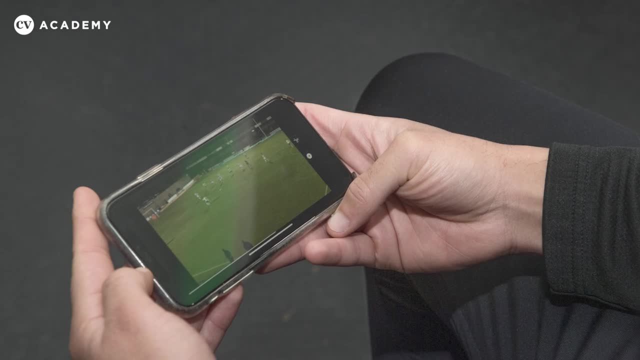 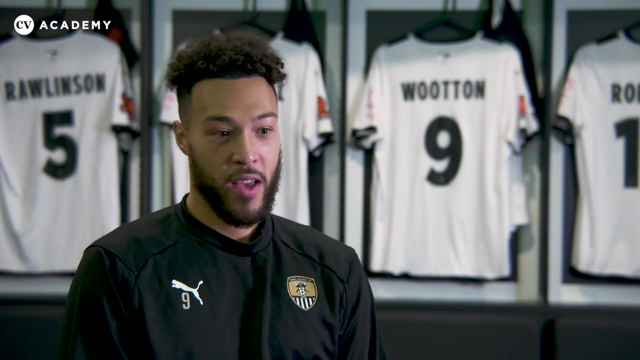 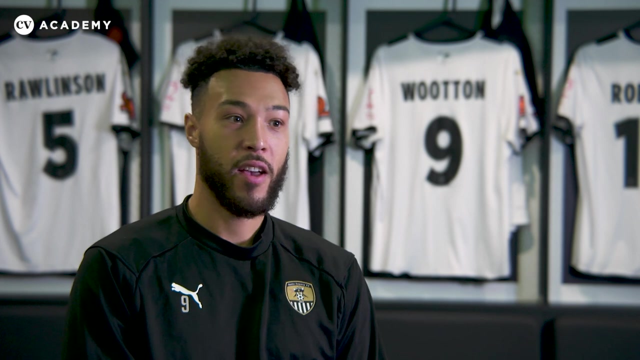 At previous clubs we've not had that. You're either having to go or asked to watch this, whereas Zhao- we've got a good relationship Every player has with him. He'll know what to send across or what we're working on to improve, to add into that area. 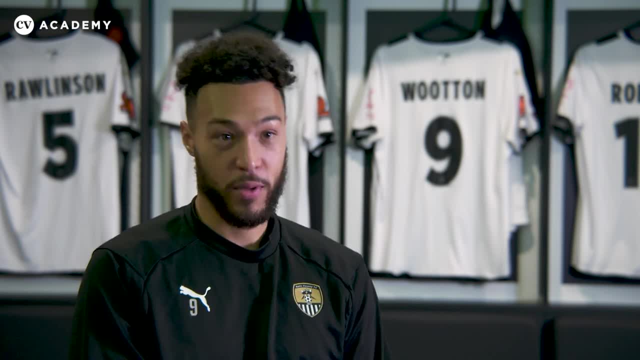 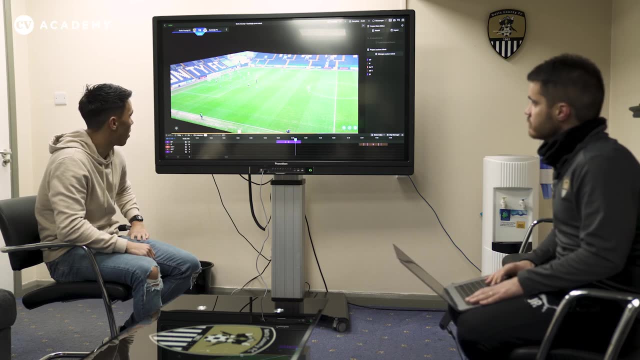 But everyone gets along great with Zhao, So it's easy to go across to him and say, look, can you help me with this, Or could you add this into the clips? You'd obviously pull him on what you would need, So some lads might only want a snippet of it. 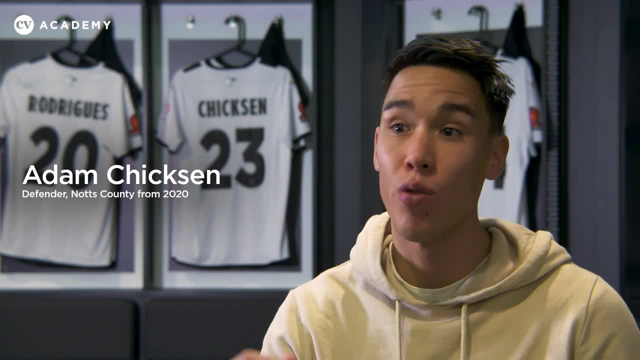 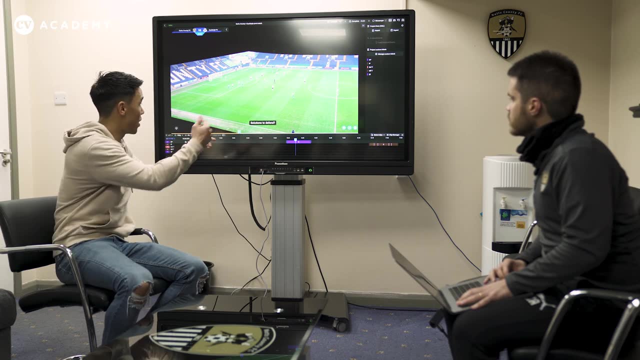 The best bit of analysis that will get them to the performance they need for that weekend. someone might want extensive. I want to know every single thing about X, Y, Z about this player. So it varies very personally, I think, when you get with Zhao on how and what you want from it. 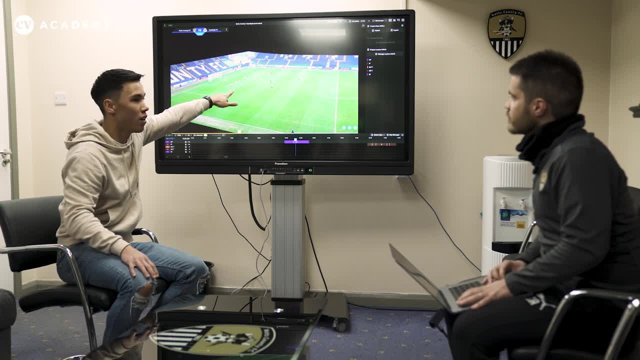 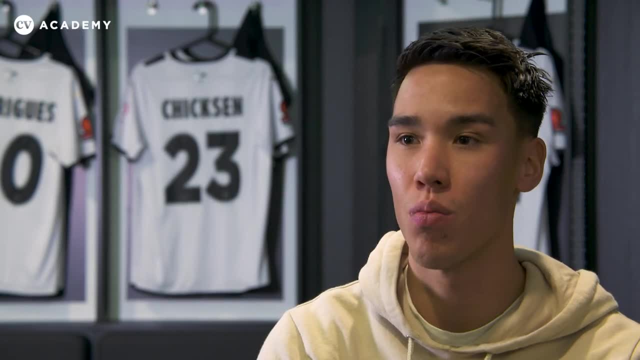 And because the programs are so good, now behind it, he can tailor it for you and the individual to improve. Without seeing what you're doing, you don't know how you're going to progress, You don't know what to progress in And with them being able to. 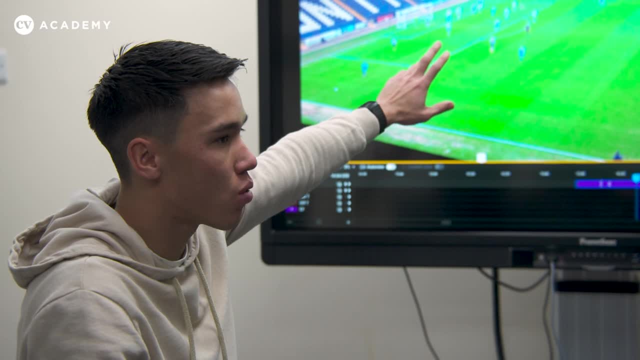 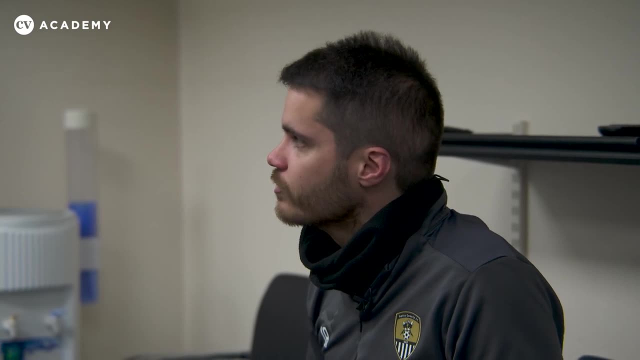 Analyze it with you and give it a detailed reaction of what you're analyzing. I'm learning stuff at 30, which I'm happy about. If I'm going to stay ahead of youngsters coming to the team ahead of everyone else, I need to know that I've got these tools available to use. 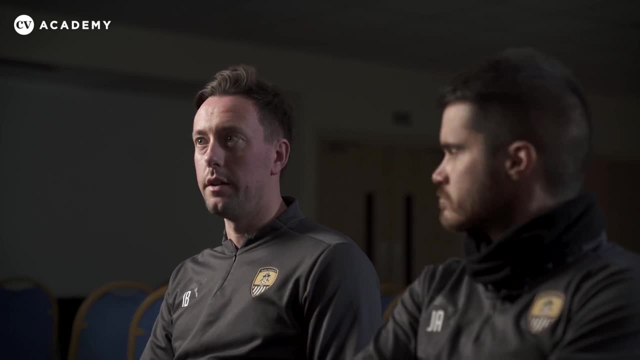 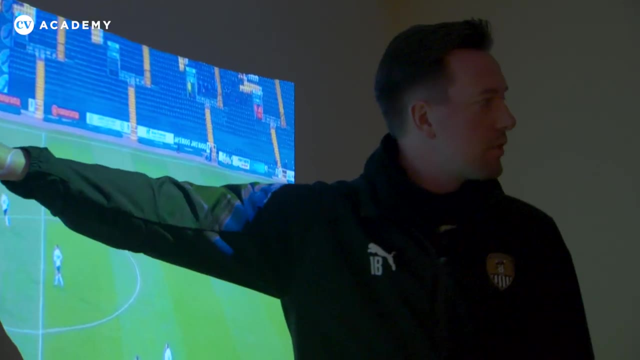 I came into first team football about eight or nine years ago now, and the technology has really evolved since then. Monday night football graphics that were there a few years ago are starting to become much easier and much more accessible at probably a lower cost. 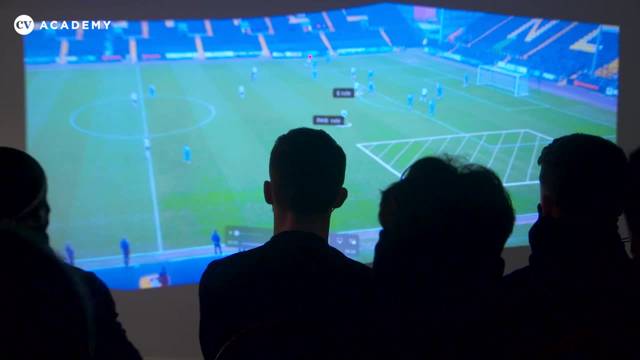 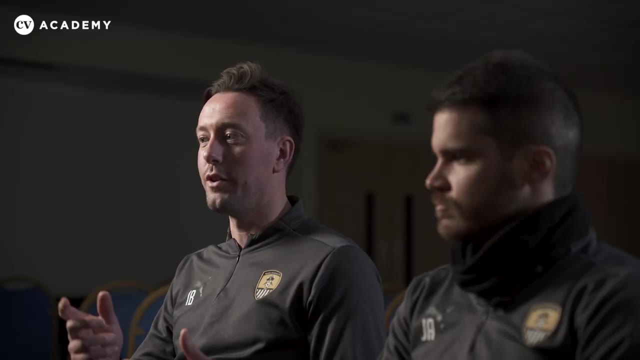 So you can make the visual aids for the players so much stronger. We all analyzed it, even years and years ago, before this sort of technology, The old school recorder and fast forward and rewind was there. Everybody was looking into the game to try and get a margin. 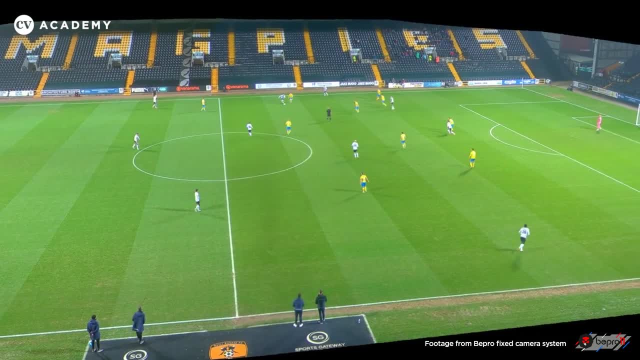 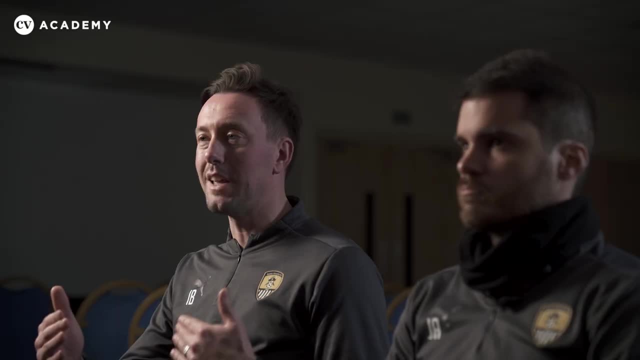 But I think it's become more accessible, quicker with the feedback loops you know, with filming the games live at half time. One of the most important things is like Zhao can come down and give me instant feedback, quick. Maybe there's three or four common trends that Zhao's picked out using the B-Pro cameras. 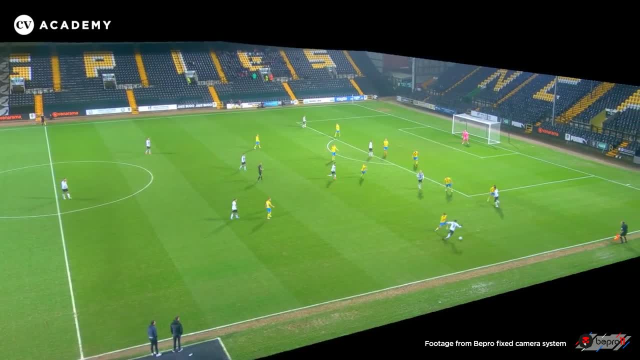 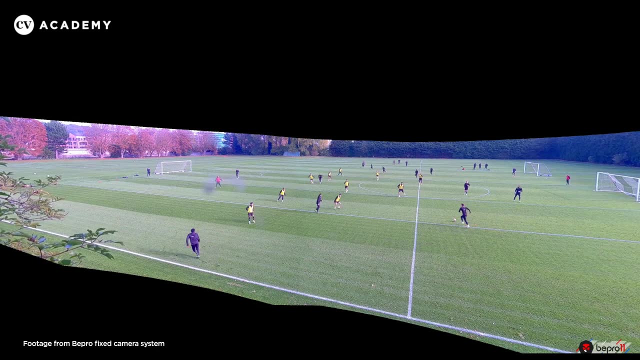 and he can come down and we can review that in depth and then go and deliver that back to the players at half time. I think that's a great asset to have. We can have the same on the training ground because we're filming it. 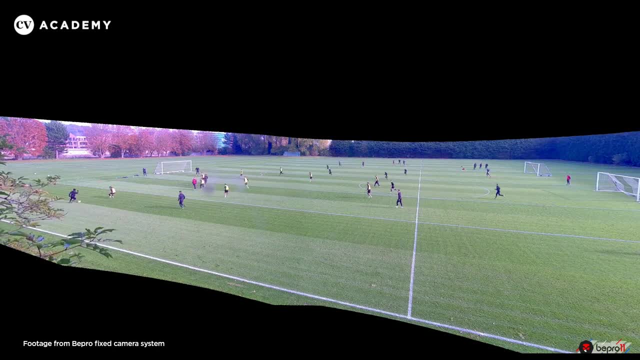 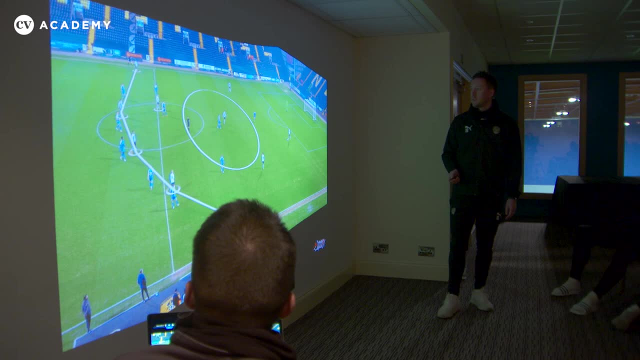 So I just think that it massively is kind of sped up and gave more depth to the coaching process. I second all of that in terms of technology, for sure, And then the knowledge actually, I think, increased in the past. What 10 years. 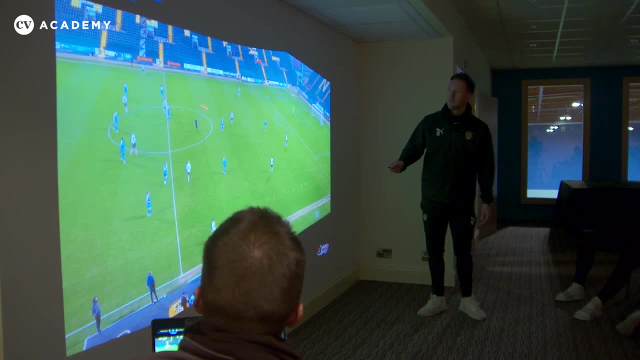 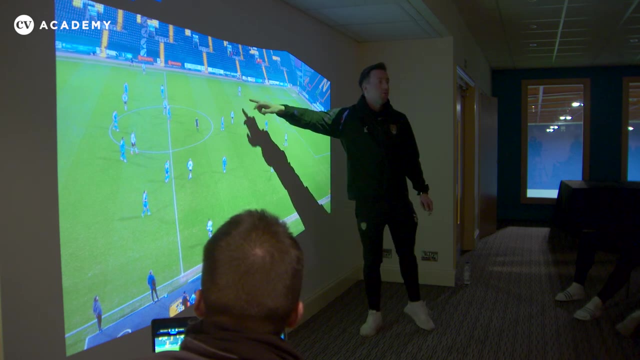 And there's a lot more people and a lot more knowledge available. So I think that's improved analysis to a good extent, And then it's improved players experience as well, because we're giving them a platform to. this is what you do specifically to have a good game. 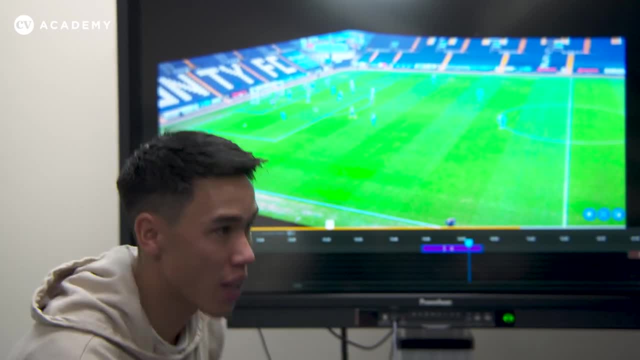 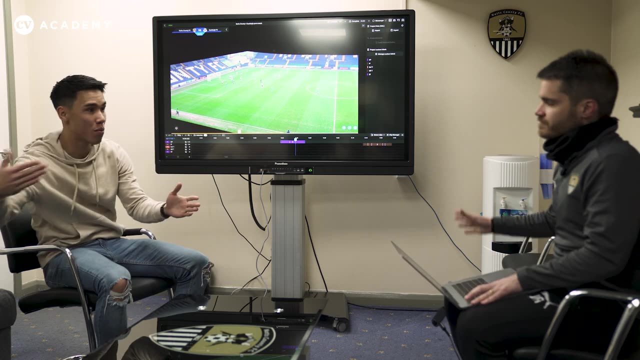 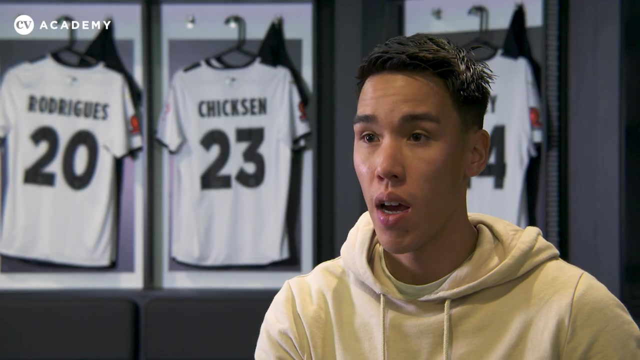 And I think that clarity as well has improved. It's been a massive change because you have to become more of an intelligent footballer, With the amount of that can be analyzed on the pitch, training, pitch, to the games. you now have to really go into depth and start using your brain more. 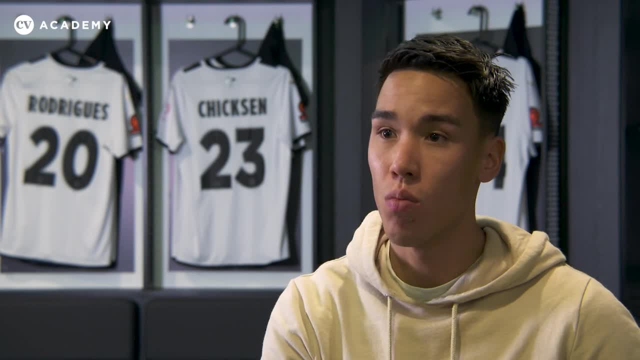 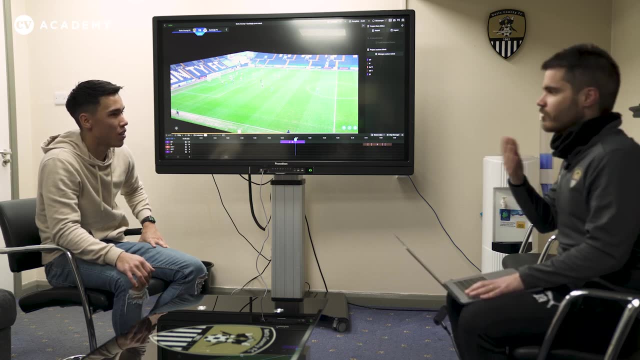 And that opens up a whole different level of progression in football. So you're not just being told it anymore, You're being shown it in five different ways. So it's then. are you capable of moving with the times? for myself, staying with it. 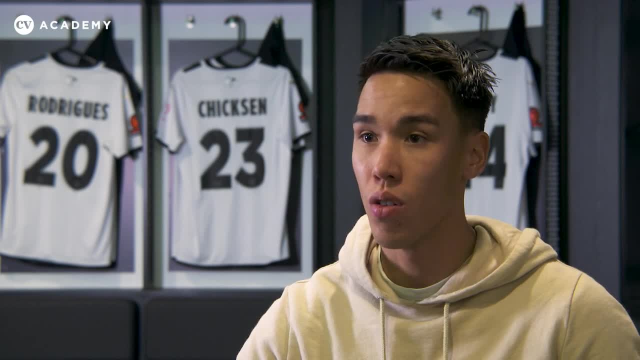 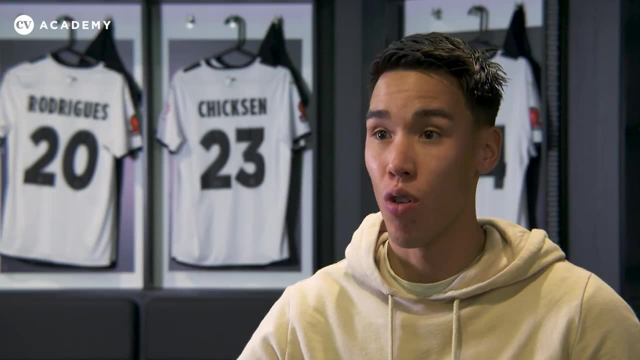 Or are you going to fall behind and the young lads going to take over? So I had to take my own readings off. it mentally pitches as I was growing up Because it was so much harder to recollect from taking information from training or all games. 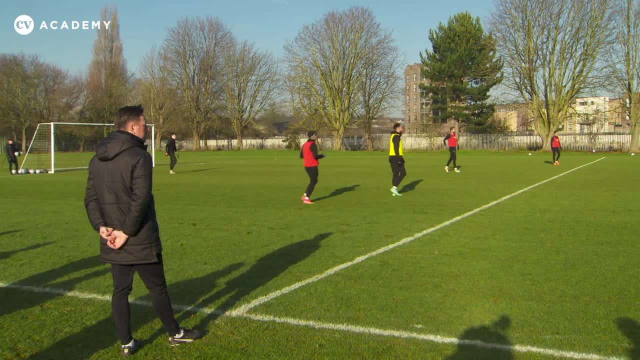 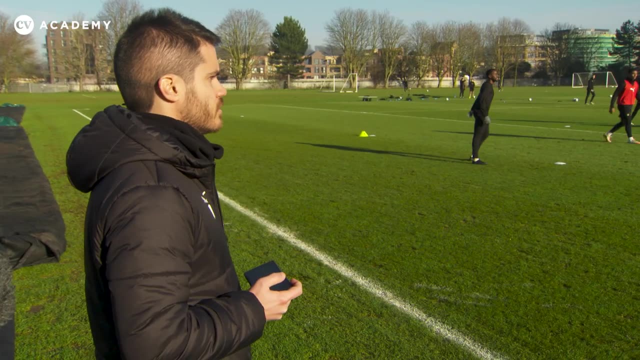 because it just wasn't advanced enough at the time. Years ago I went into clubs and they were needing three, four, five analysts, And they were. we probably getting that kind of quality of work with less personnel now, which means that you can go further down the leagues with maybe less finances behind you. 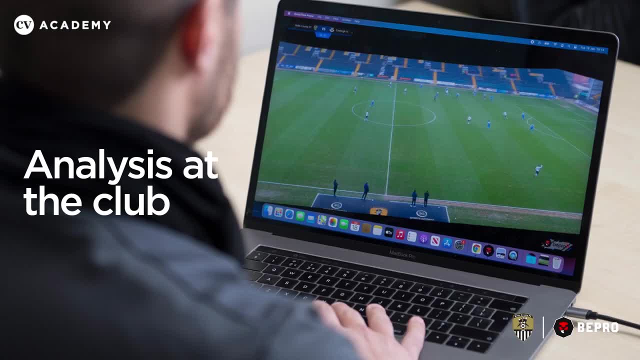 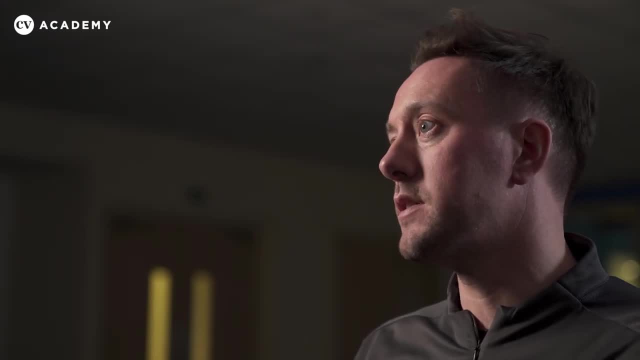 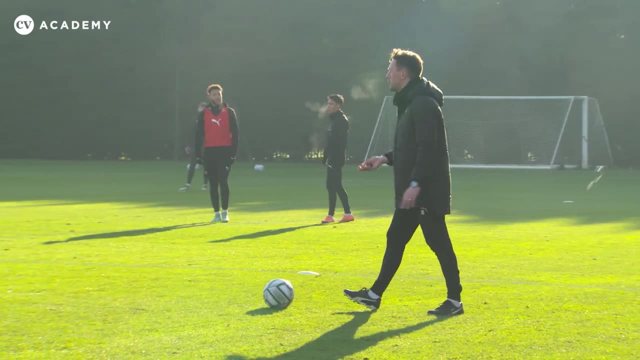 but still get good quality analysis done On a week, On a week, On a weekly basis. some of the we have big group meetings, obviously with reflections of last game and then opposition analysis for upcoming games. So they're normal. But on top of that we probably we have small group meetings. 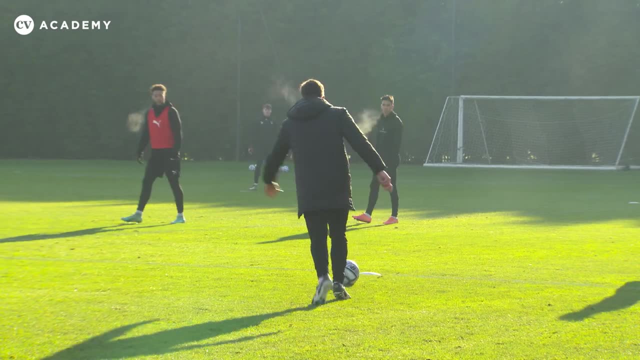 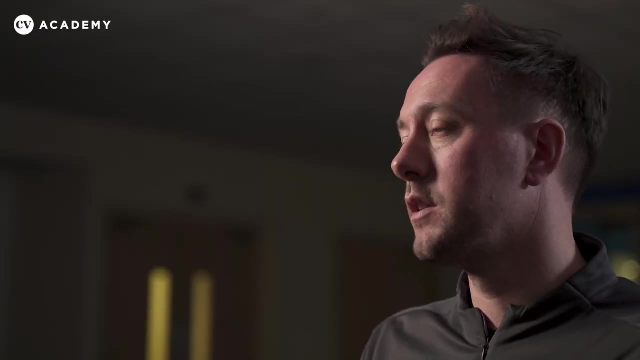 So unit meetings, defence, midfield attack, But then on a daily basis we will- myself and Jao, the analyst, will- look at training. We'll go back through the training sessions. We'll maybe clip bits of that to be able to send or show players the next day. 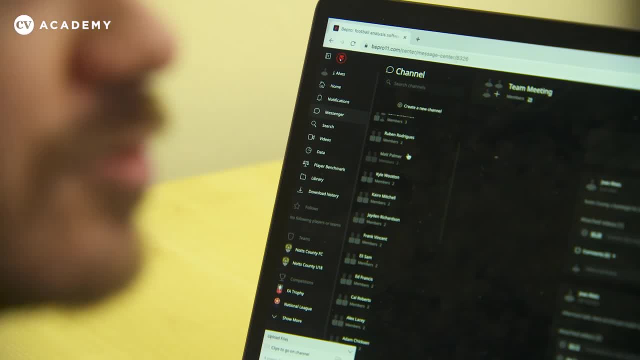 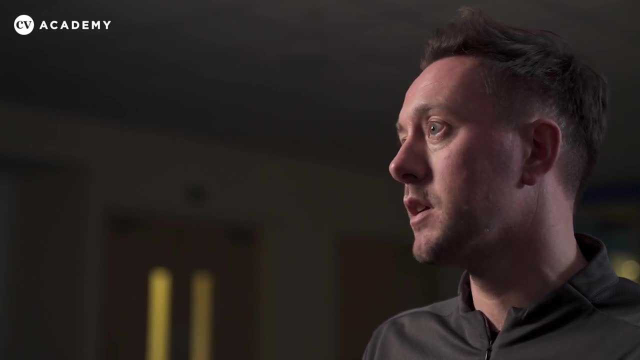 And also use it in one-to-one meetings. both myself and the other coaching staff on board will also be active in terms of clipping certain players positions, roles, responsibilities, just to try to break the game down and give as much feedback as possible to the players. 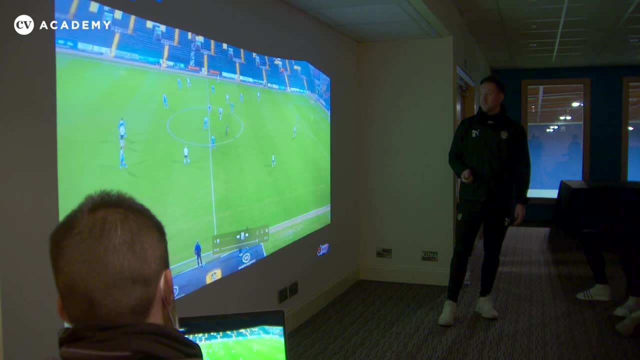 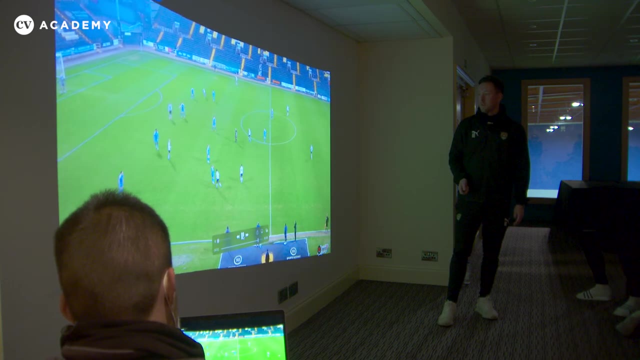 So they're not coming in and the only coaching they get is on the pitch. There's a lot of information that they get in and around the actual training itself. Probably, overall, we use more time than we did before, but that's because we've now got the training ground cameras, which we didn't have last season. 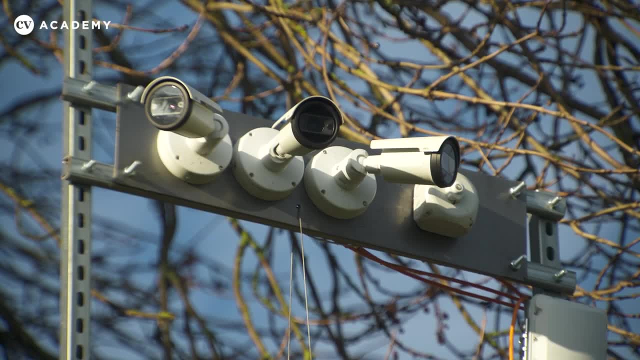 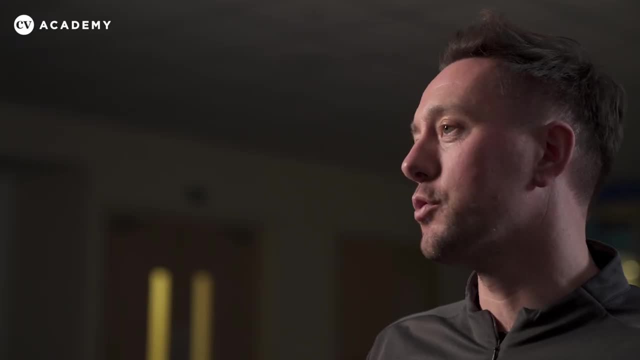 So we introduced them, which obviously increases the workload. It's a bit low for myself and the analysts, but it does give us much better feedback loops for the players. So I would say our overall time we're probably using a bit more than we did last season on analysis. 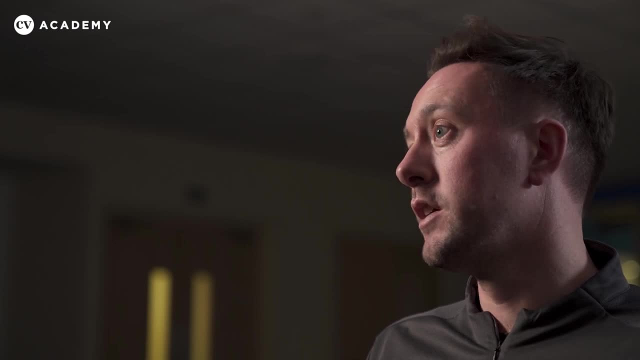 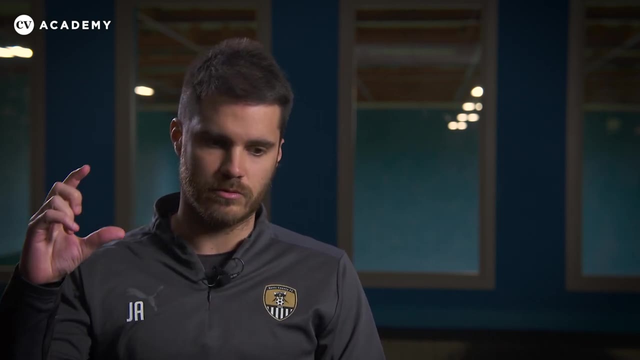 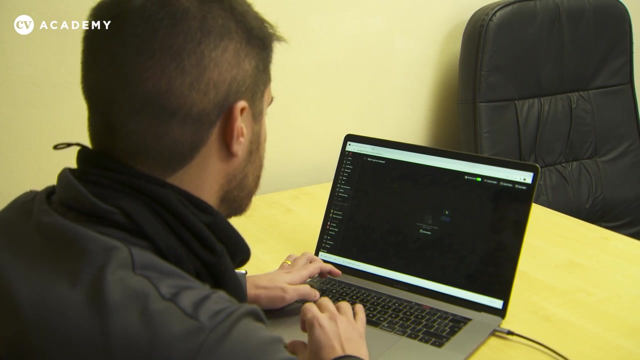 But the quality of the analysis that we can do in the shorter time is much higher. It's a cycle, So I do post-match after a game, So we go day-to-day. so we'll go before the session. We'll get together, we'll look at whatever happened in the game and what we want to push to the players as a group. 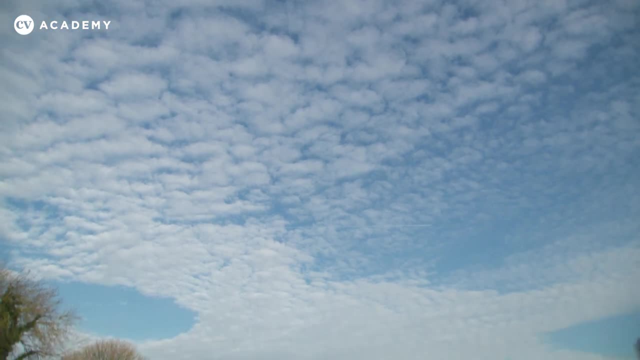 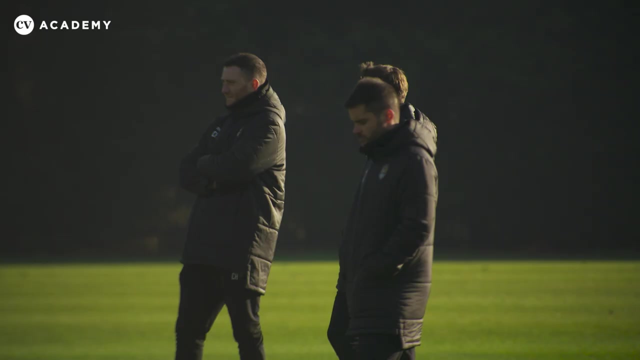 Then what we want to push to the players individually. I'll then go to the training grounds. I'll have a look at what's being done. I found it very helpful to know exactly what's being done in a training session, because that blends in with what we're trying to do as analysts. 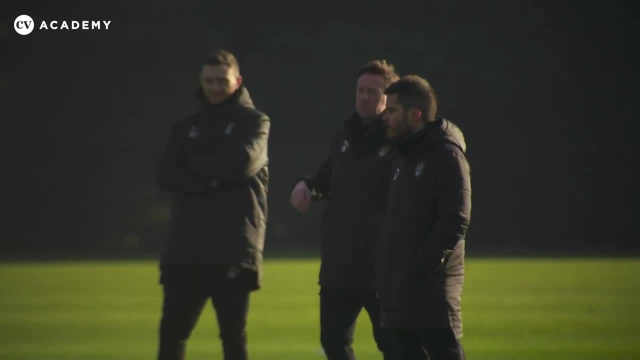 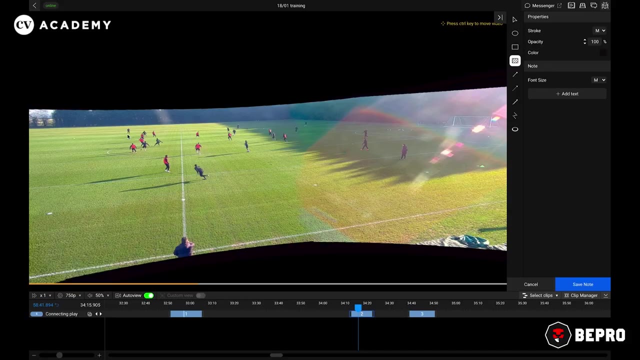 I'll get the recordings done, then we'll come back. We'll review training whenever there's interesting tactical behaviors. I'll start then looking at opposition analysis and pushing out bits with individual players. And again, it's a cycle, It's constant feedback. 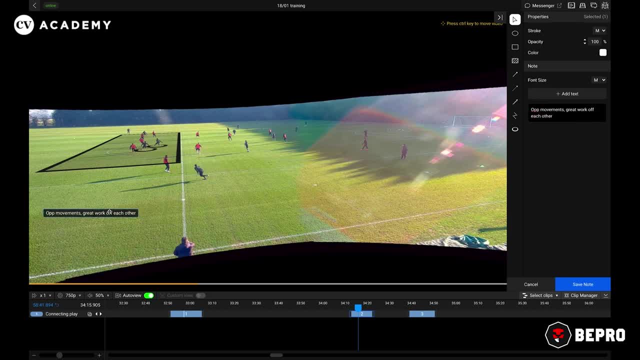 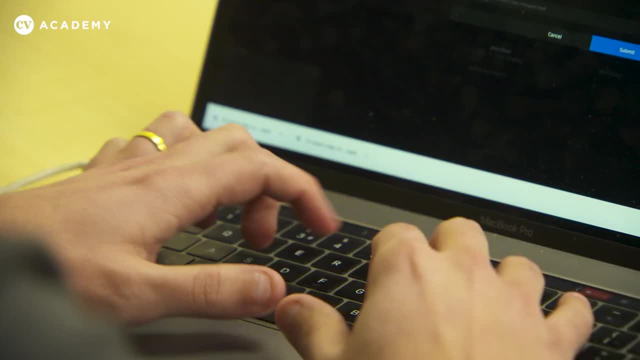 And it just goes: we've done this. If we've done well, why was it that we've done it well? So we try to give them that platform. that base of this is why it's good. So then it becomes clear as a behavior what we want. 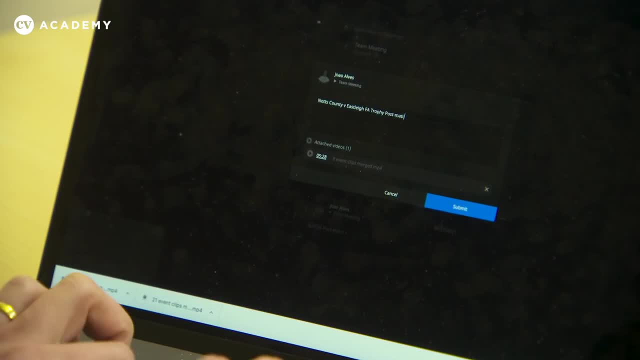 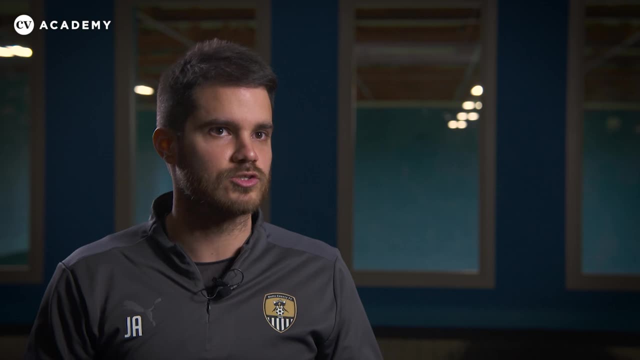 And then same with when it's bad. If it's bad, why is it bad? If the game starts to stretch, what's causing that to stretch? How can we correct it? If the game's nice and compact and we keep it as we want it? 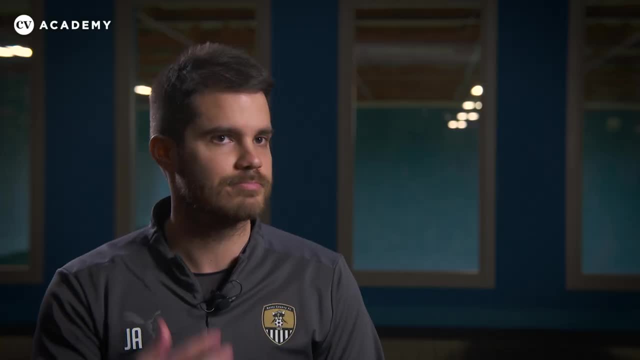 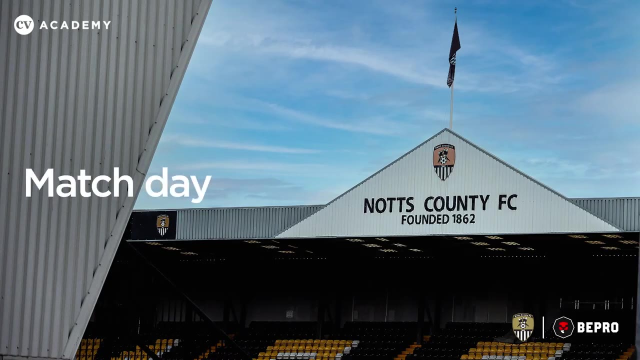 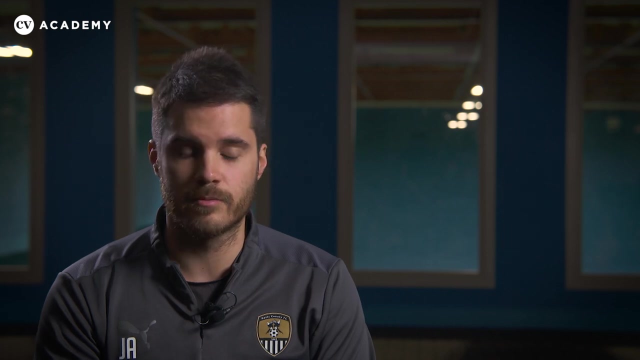 then what's the reasons for that And what's impacted their structure And what's given us success? Depending on what we decide, we put some content together for the players before the match. So now, 45 before that's when we announce the lineups. 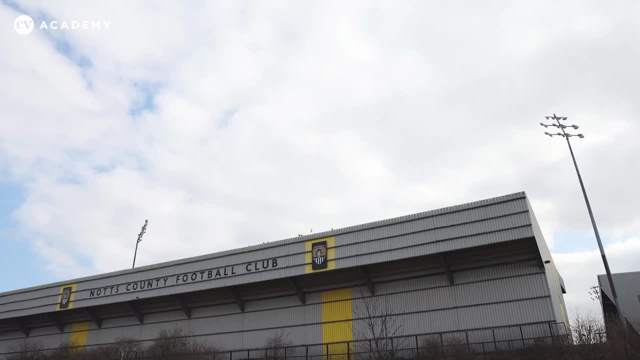 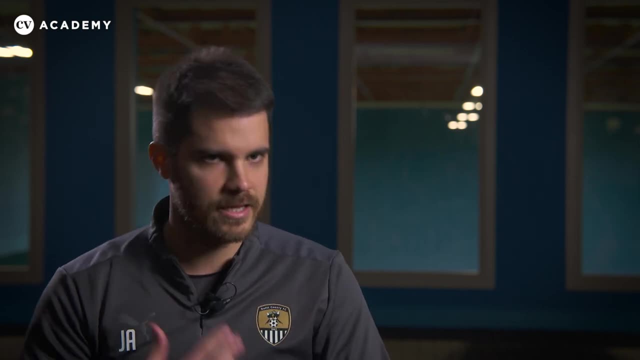 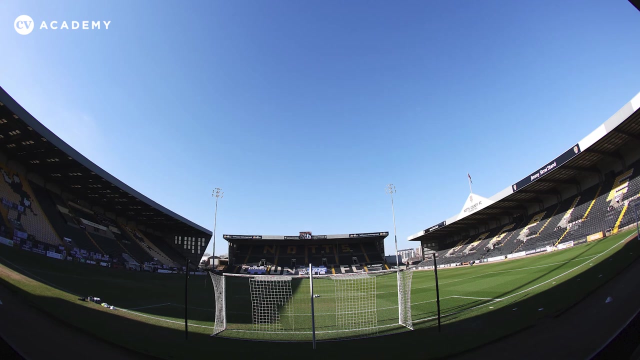 So we'll have that on my laptop ready to put in front of the players. Then it's a bit of a waiting game until lineups are announced. Then it gets a bit frantic with trying to understand what the opposition are doing, where we can start to kind of predict and assess where are we going to get joy. 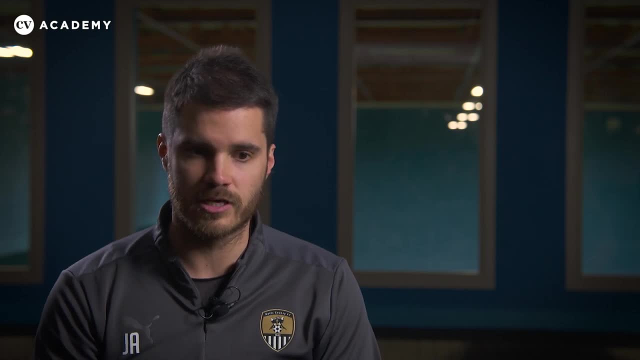 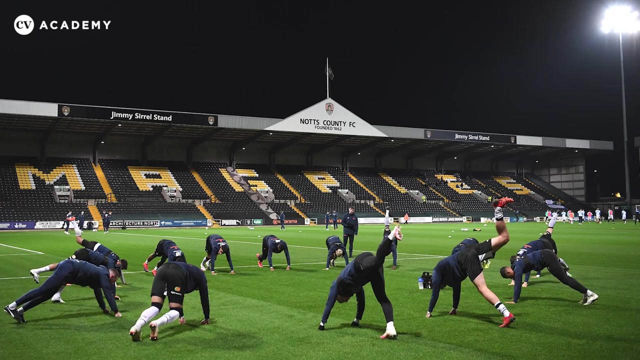 where we're going to get troubles, I'll put it up on the board so the players know. I'll give them a bit of information in between, so the individual bits that maybe didn't filter through to the group meeting I can just go through. sometimes good practice is to just give an example of a clip they've done in training. 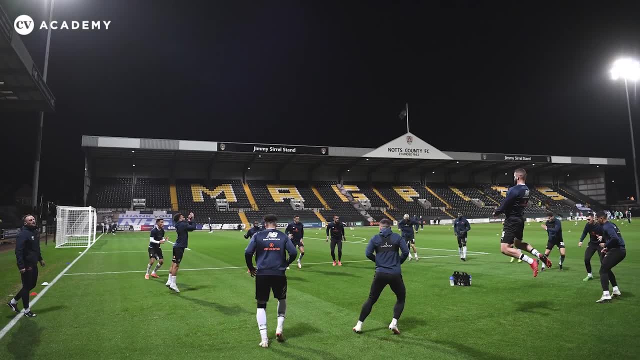 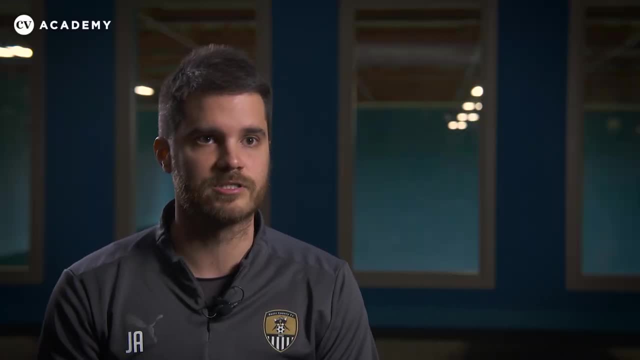 or a clip from an elite player and then from there go up to the gantry. I've got the radio so I can just radio down anything I see the guys can radio up anything that they're particularly interested and I can just clip it straight away. but particularly half time we bring it down and see. 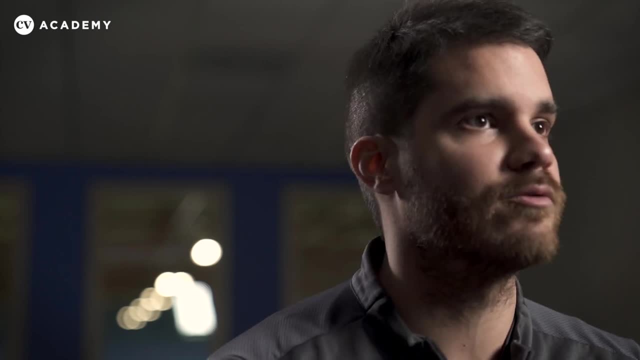 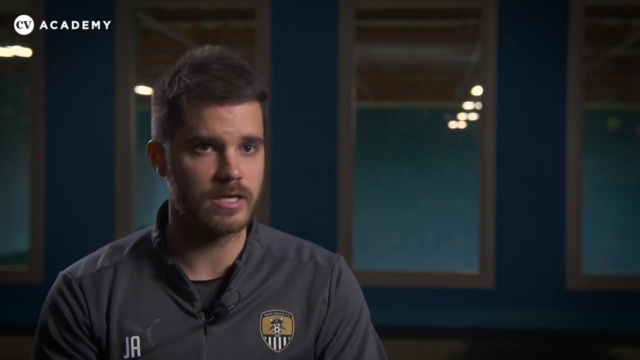 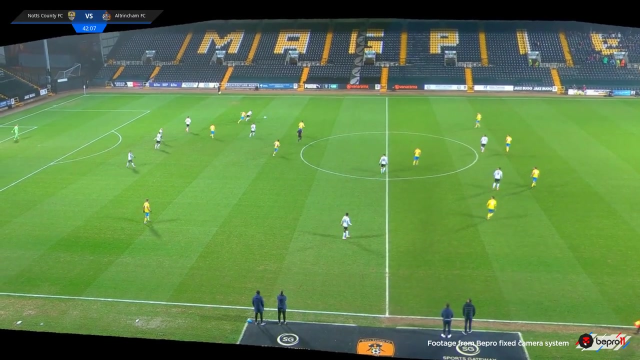 what? what? I give them a better, clearer picture of what's going on. it's tricky to see it pitch level. then we'll go into the changing room. the gaffer will speak about the key messages that he wants to send. then again we'll have an opportunity to put in some smaller bits in front. 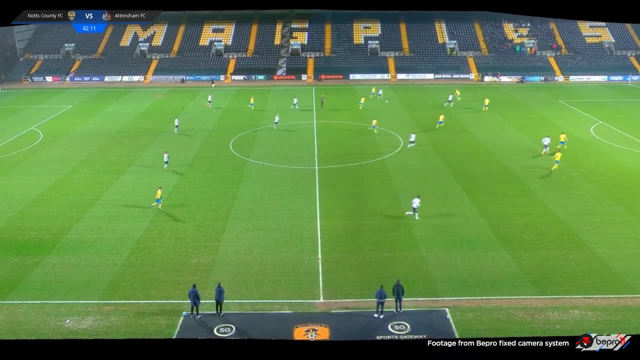 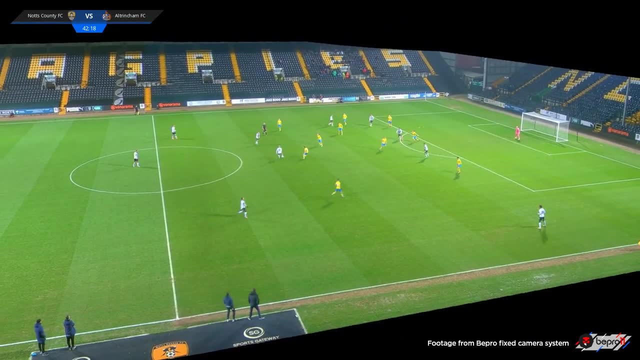 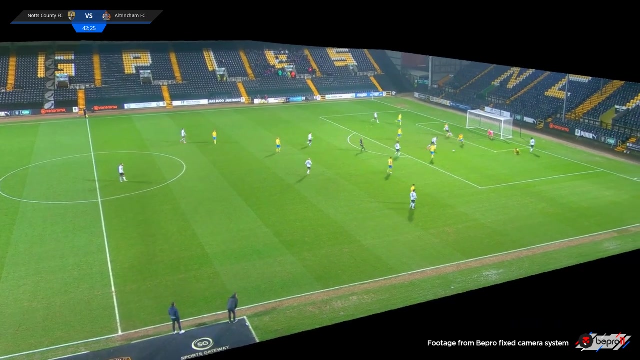 of the players with a picture, which is great. I think that gives us actually a lot of buy-in. I've I've found, when we don't have video that the message can get lost. the ability to look at half time with the, with the quality of the camera that it gives you and the immediate feedback that it gives. 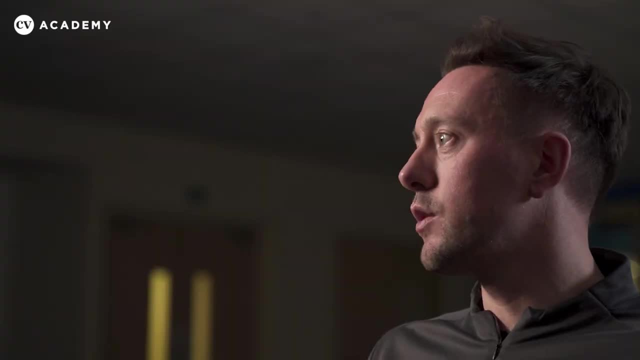 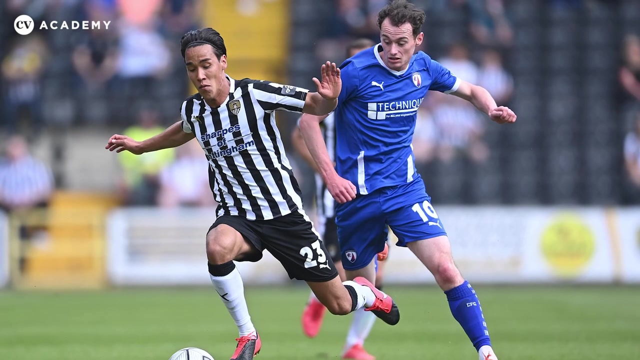 you. I think is really important because as a coach you have a small window at half time where you can make those changes and be proactive and really get messages across. when the players are out on the pitch it's so hard to get quality of message across. we have the cameras, the wide lens vantage point. 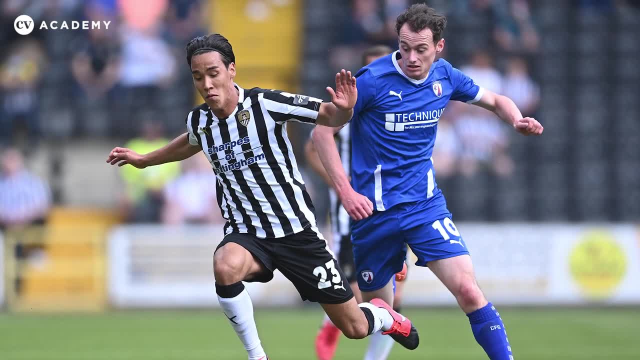 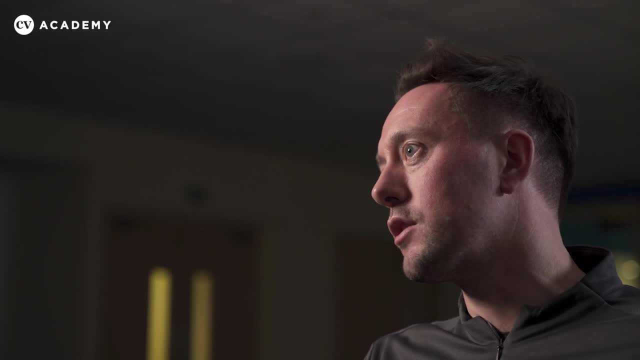 being able to clip things by the time I'm in at half time. you know you're pressed for those minutes, so as much feedback as I can get at that half time is huge and when you have that 15 minutes you've got to use it really well and I think B Pro certainly gives us the feedback to allow us to be. 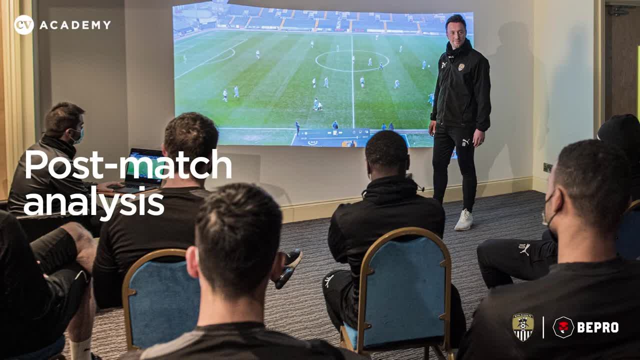 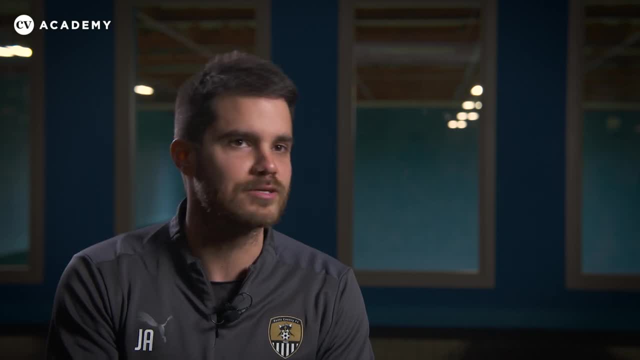 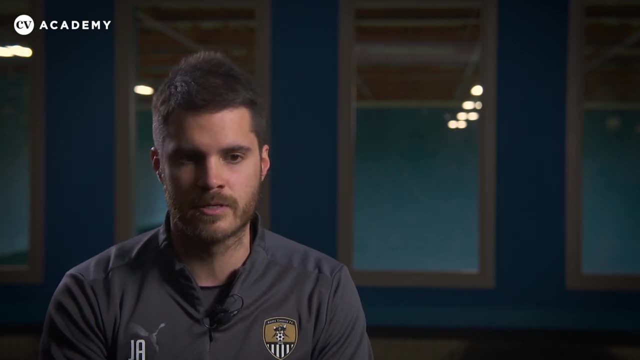 more efficient. at half time I try to affect the outcome of a football match- I probably don't as much, but to have that option and to try and to to show that at half time or in game, but the other one, I think this is the one that really come it's natural to me and it 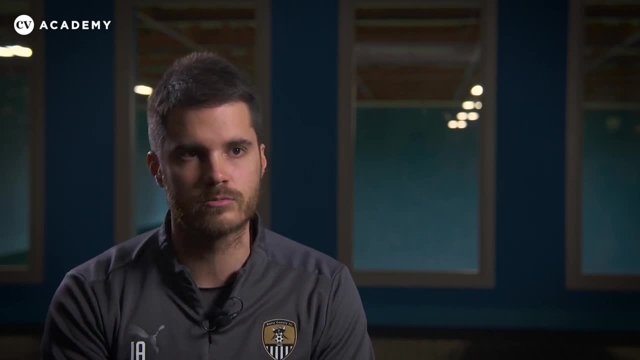 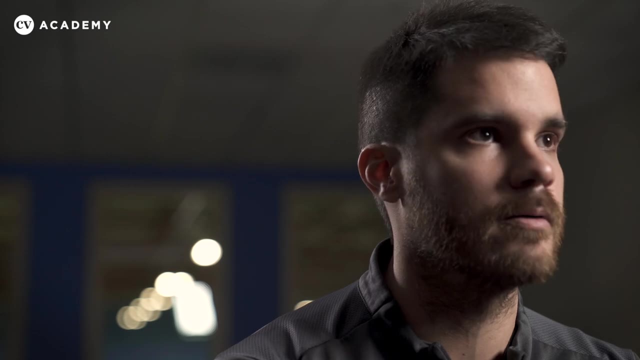 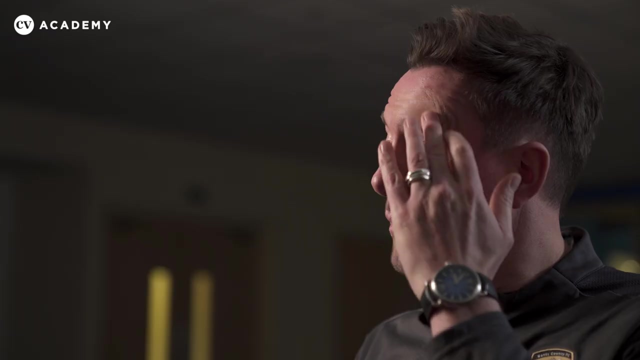 happens. more is the reflection and the review of the game. so our post-match: why have we had success? why were we unsuccessful? what were the factors? how can we get better? how can we assure that we keep at it? myself and the staff tend to watch the games back anyway. 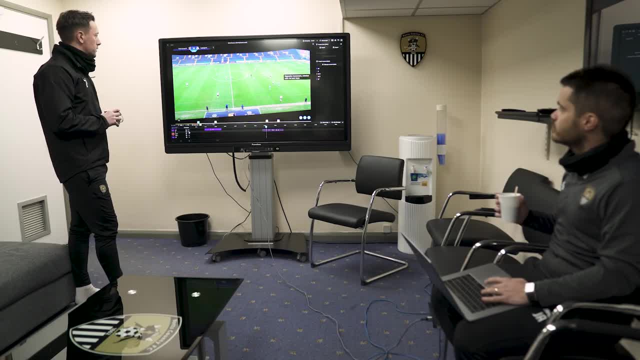 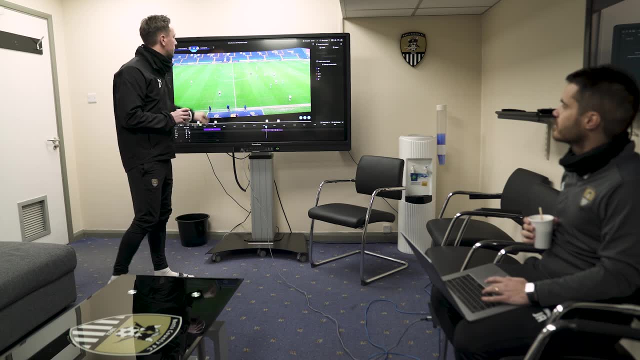 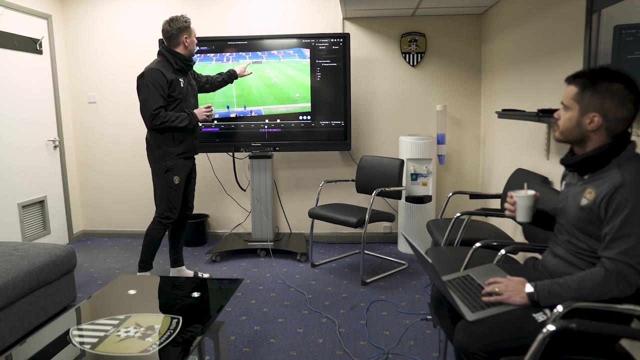 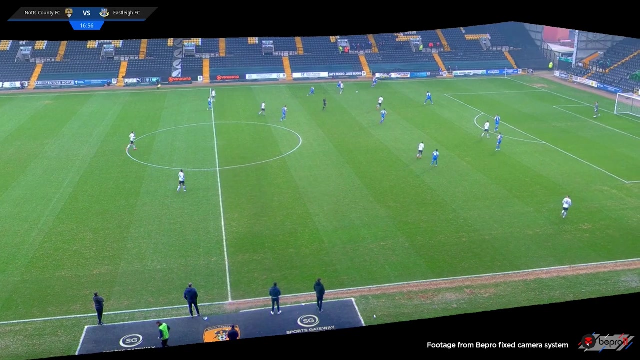 of course, the next day, but then when we come in on the Monday morning, Zhao will have will have clipped it for us, and the more we've worked together, the more he knows what sort of things I'd want to look for, and then he will present to me what he's seen. so breakdown of what we do in possession, out of possession, any other trends within the game or problems that we might have had, and then that could be 20 minutes, half an hour, but then we'll we'll clip that down to a more manageable amount for the players. 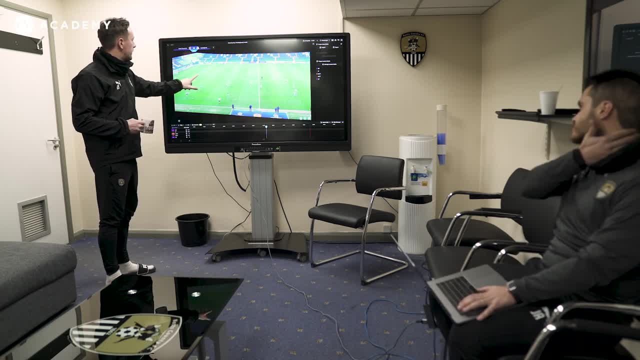 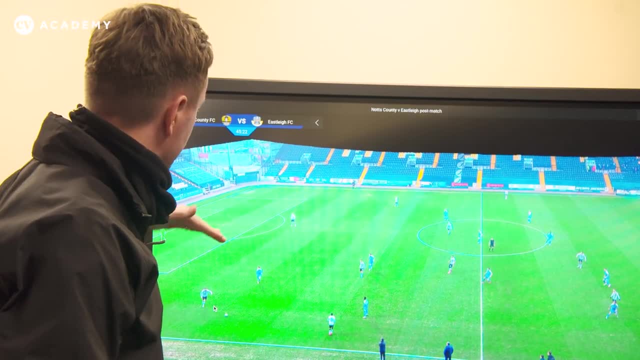 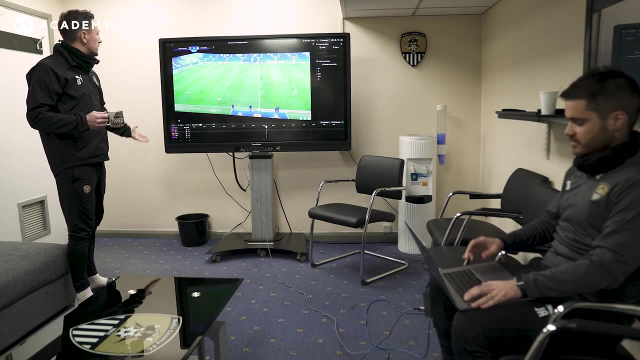 for me, stop the. this is no brainer here. here we just come out and all the spaces on this side, but we've played three, four passes all on the same side and then we end up doing this one. This is what you're talking about- body position, cause I've heard he's it's body shape is just to go look. 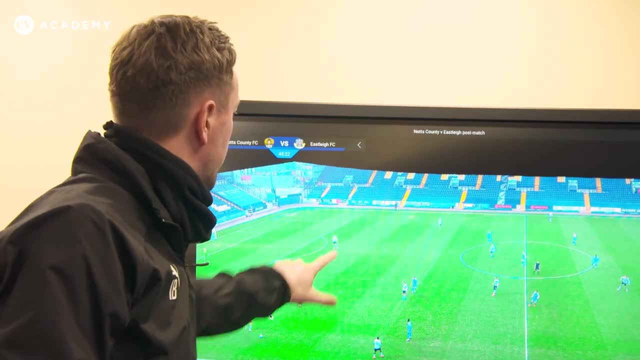 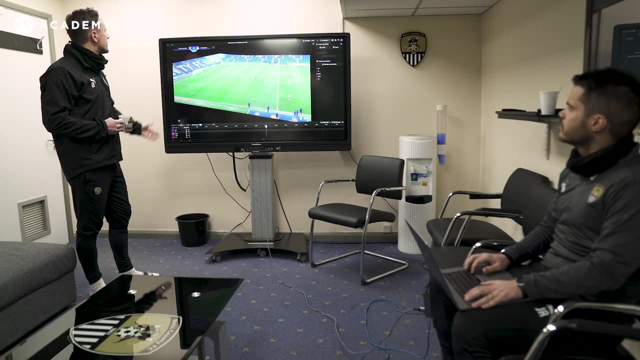 just need to turn open up, play there, come out, but then we just do that. yeah, do you want this? Yeah, I think so, because I know it's on half time, but we can, You can control this moment. There's still two minutes left of this half. 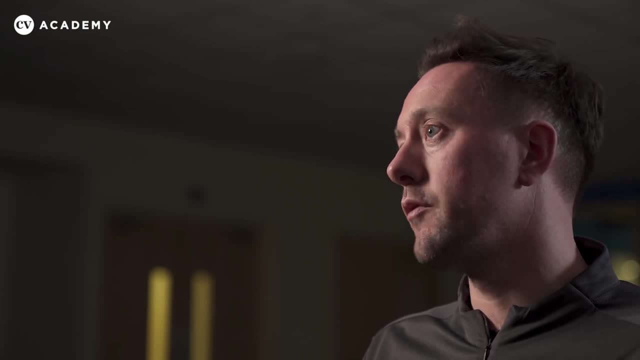 Maybe we'll end up showing the players up to 10 clips, but we'll try and find a common theme and we'll try and link it to the next game so that it is consistent with the messages that we want to put on the training pitch. 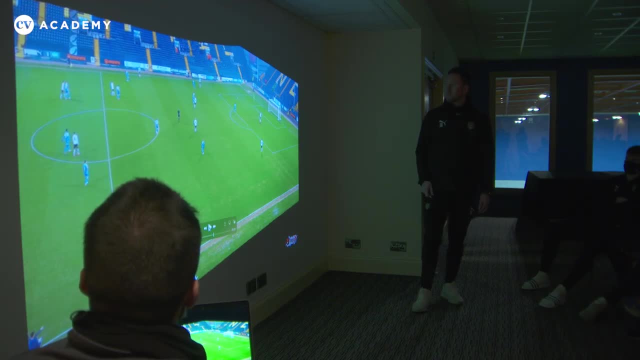 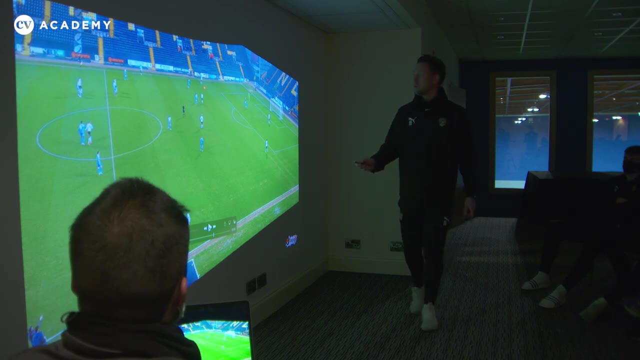 What do we think to this build-up? Where's the ball got to go Out left all day? I think that first pass, Connell, is too soft. I think you can wrap that back to Sam so he can take back foot and get out. 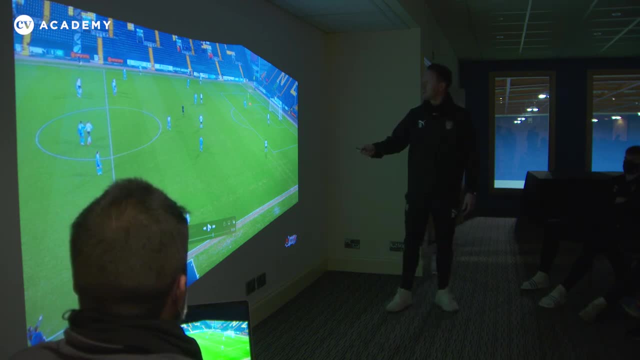 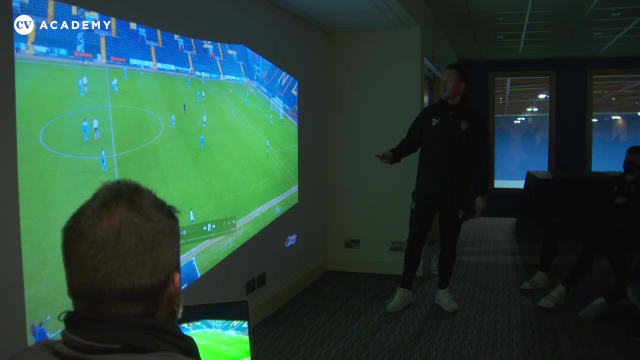 But even so I still think back foot. This is the pass. here We have to push that. we can play this pass and then we get out. Look at the space Chicks has got- and then Connell will run them off If we keep playing same side and clip long. 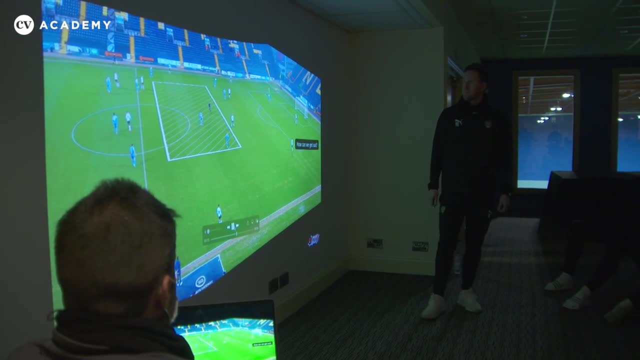 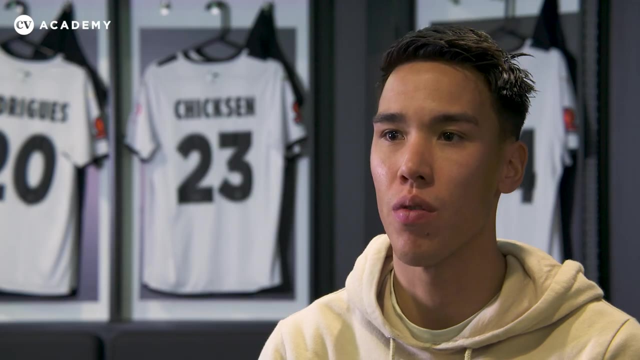 I don't think it's to our advantage. And now look, Vinnie's dropped Cal's a little high and then maybe we don't land on it well enough. in here Daryl can put on a very good and simple. I know I say simple. 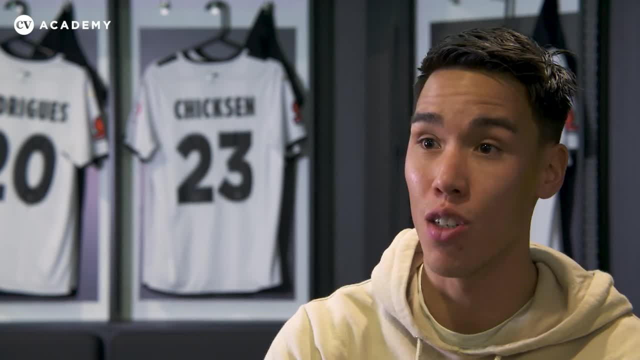 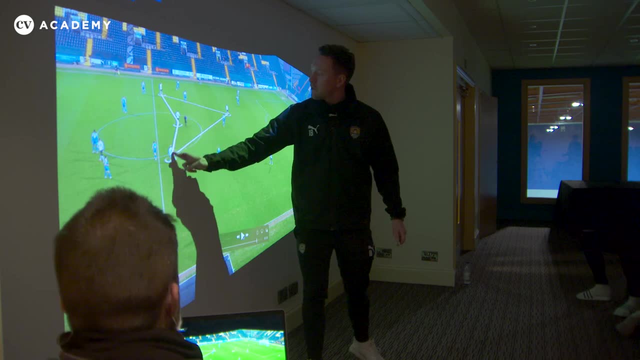 but it's very extensive what he does, But for us lads it's made simple and that allows you to process the complexity of what they're trying to do, The new sort of distances to lines, to areas you're trying to cover and protect. 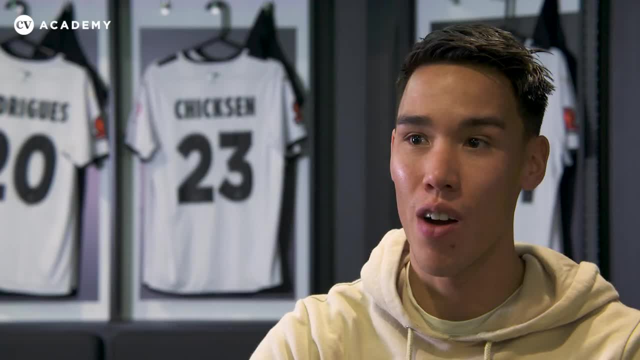 And it's something where, if you're saying it, they might not process it much, but how you're able to analyse it and put it in it's like it's quite simple. I think that's a great position, Chicks. 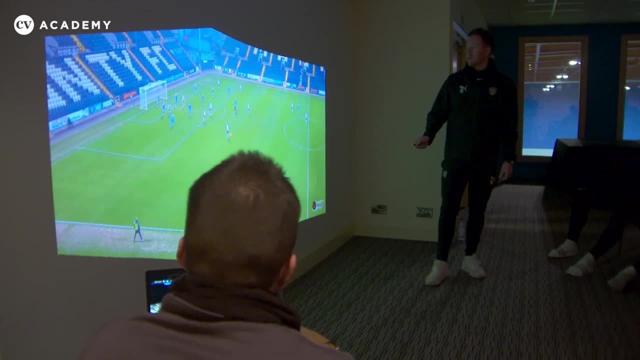 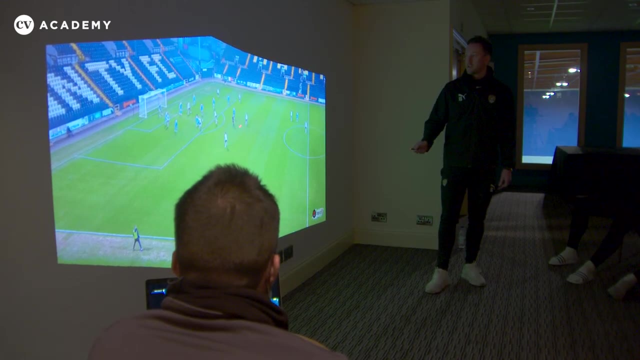 Just if you stop there, how we double pivot. now we've got two V1s, so, Chicks, you can come up here instead of you know, three versus one. come up and join there. Where's Chicks? Yeah, that's a perfect position. 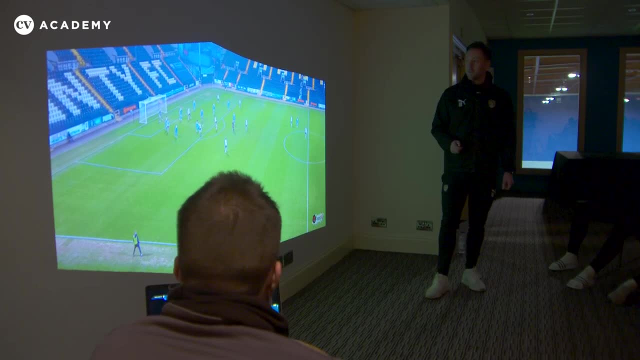 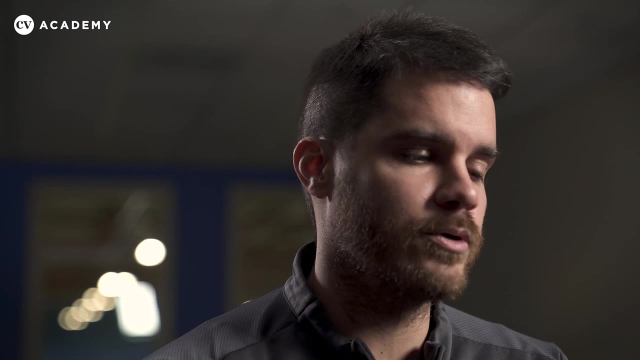 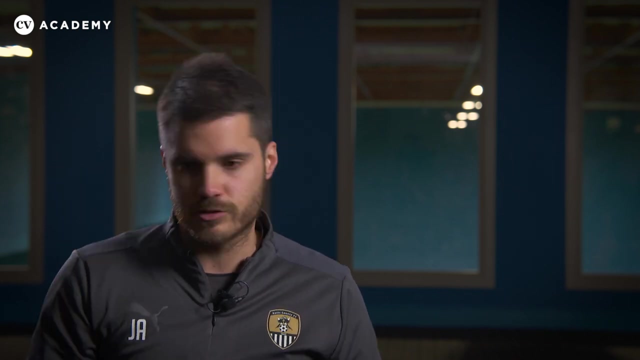 You see how the U2 have just got that everything locked out in front now With the training ground footage. what we tend to do is after the session. we'll just use that as another reflection. So we'll have the session objectives and we'll have objectives for all the drills. 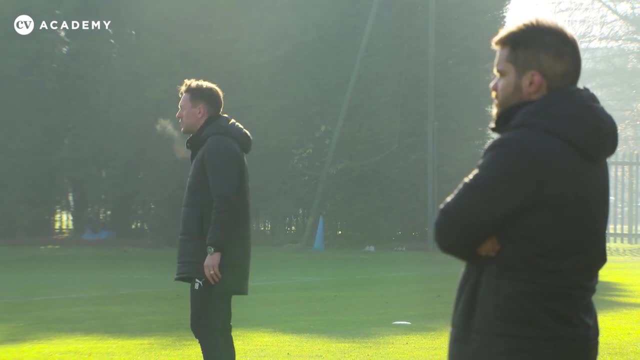 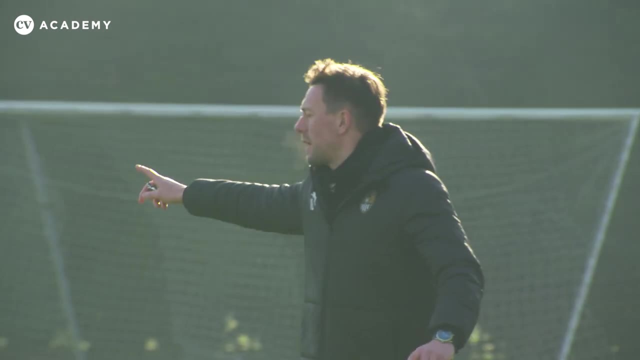 All the drills will have tactical components And we'll just like verify that those behaviours are being met And if they aren't, it's easy to just go there and identify why and start to push it out. Also, I should say we push it out a lot. 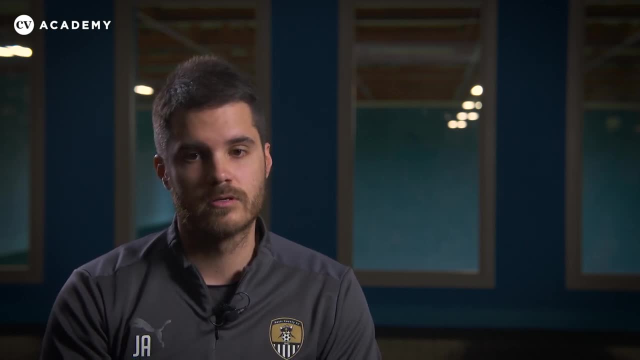 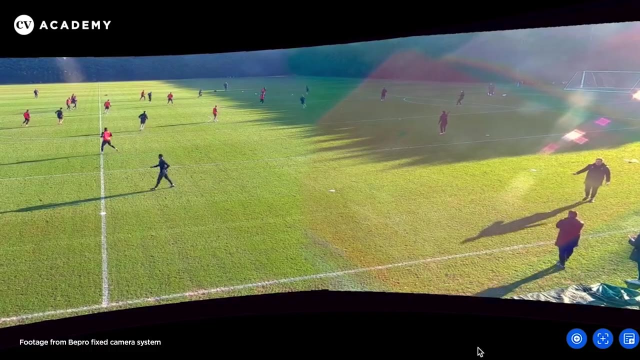 when the behaviours are good, because we feel that actually it's worked quite well for us. when we see something good, we praise it and then it starts to happen more and more. I've always liked to film trainings because I like to watch back what we're doing. 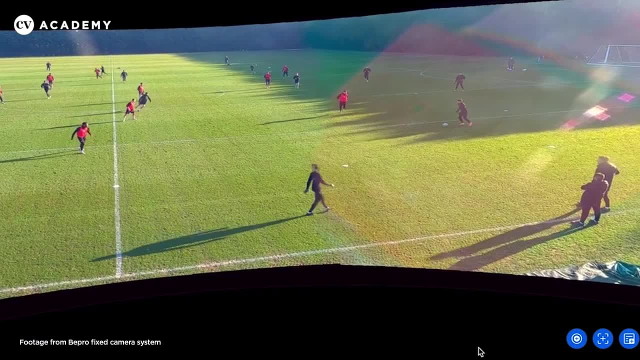 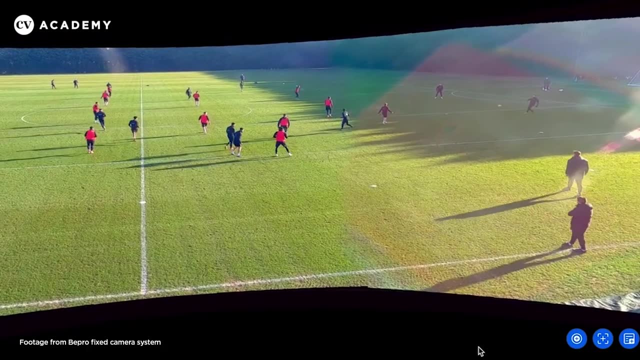 because you get to see it When you get so involved with the training. I think being able to be more reflective on your own practice is massive. I think it depends on the training that we do, Like today, when we've had the bigger area stuff. 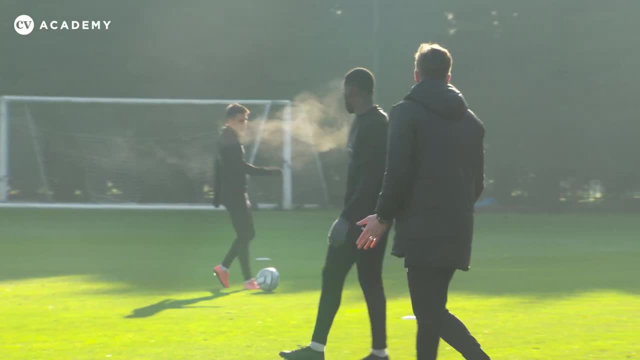 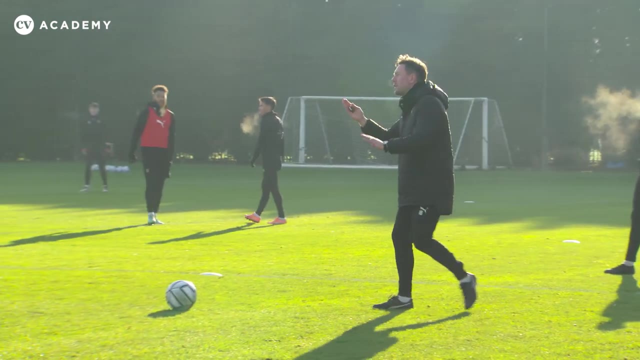 there might be some really good clips of some of the movements that we've discussed. We might just think about one or two players and key roles and after the training we can just put it on the TV. We sit down, we flick through the training. 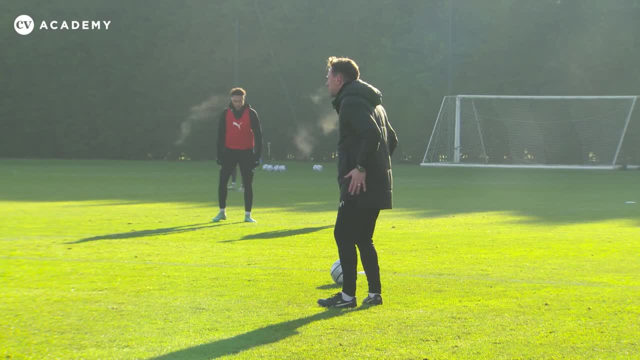 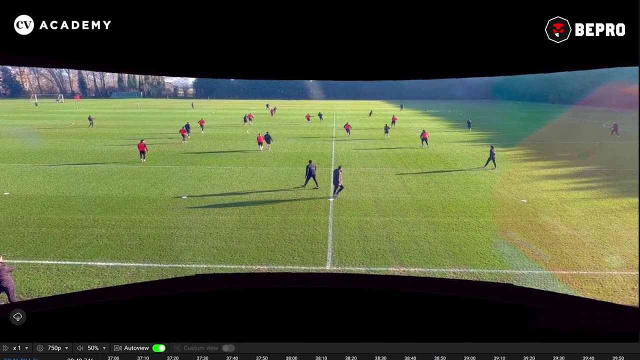 and if we see some patterns or movements or things that we thought were a problem in the session, we can clip them. Either we send them to the players with some notes on them or maybe we catch them in the morning. sit down for five minutes. 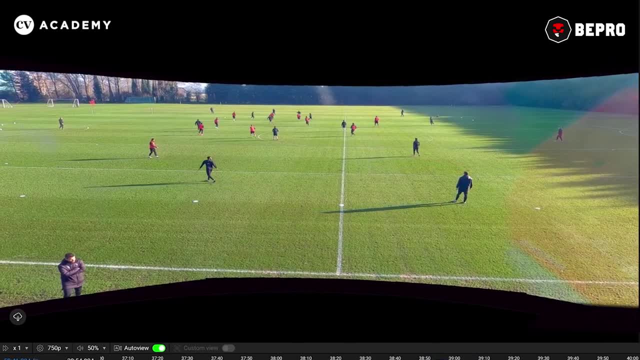 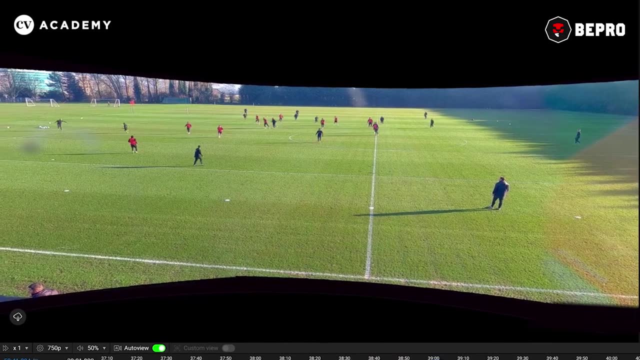 go back through their training from the day before. But it's a good process for me as a coach because I get to see if what I was coaching is correct, if the things that I think I was trying to work on in the training session happened. 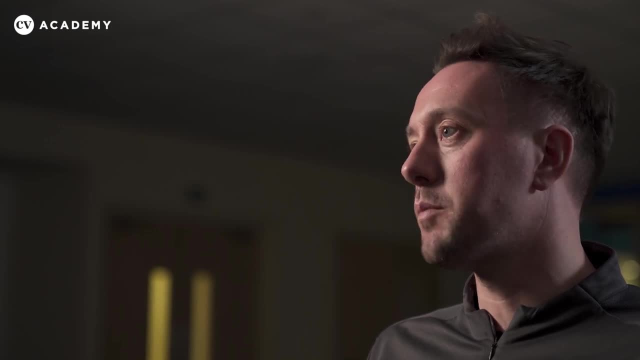 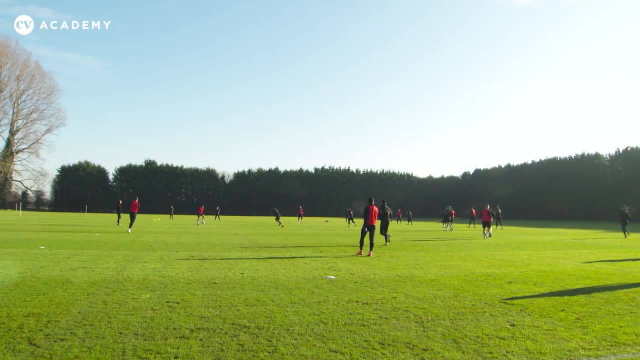 and you get to be a bit more reflective on that. And I think it also gives the players. sometimes the players are just in the session. it gives them a chance after the session to sit down and really look at what they did. Too much distance that isn't covered. 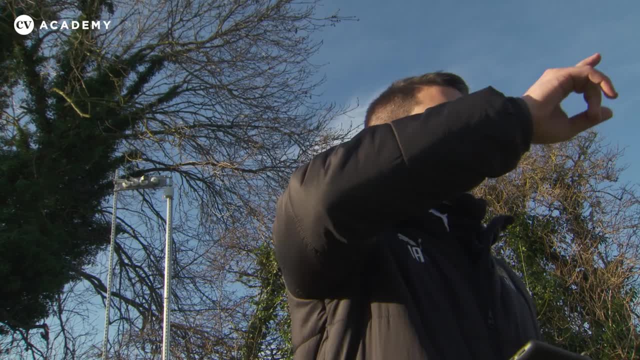 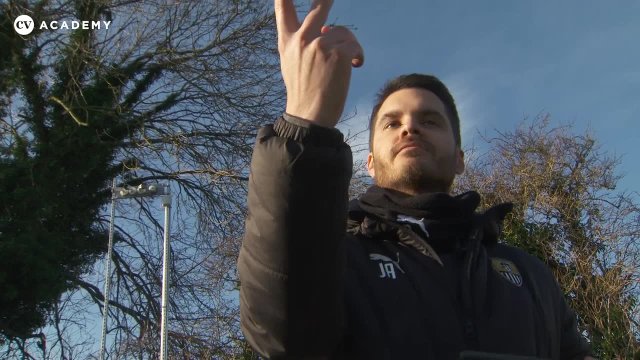 So that means that this pass needs to be bigger, And as the pass is bigger, it means that it's harder to land on things if we don't occupy the centre of the pitch. So what we need again is just to vacate. occupy all the time. 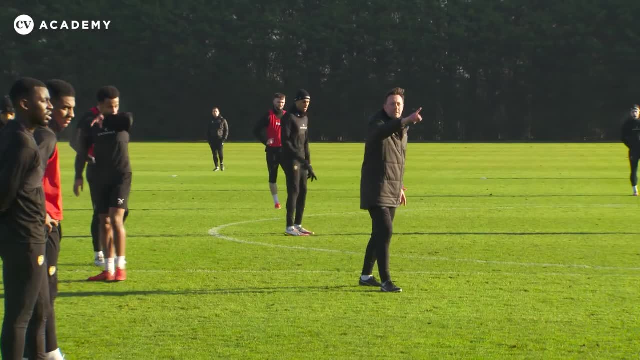 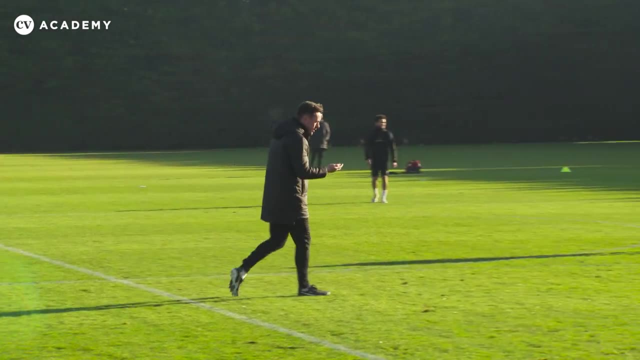 Yeah, that's what Gaffer's saying. now, There was a moment today that we've had our centre mid making a run, which means that, structurally, we're going to create a gap there. So what we need, what we need to do, is to arrive back into that gap. 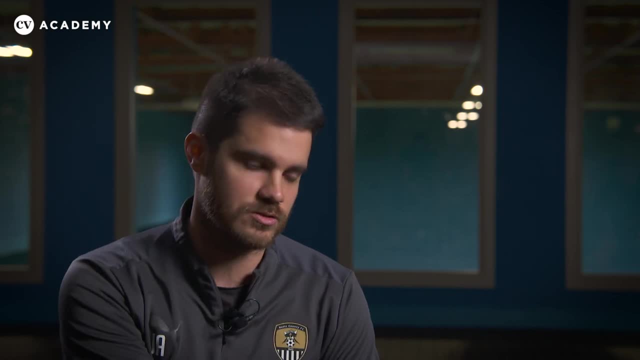 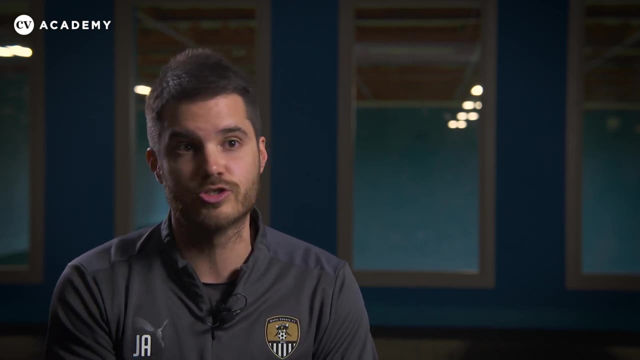 so that we're more secure beyond the ball, so that we can land on second balls and keep going, so that we can take space that's just been vacated and should be there to be taken, And, as I saw that with B Pro. 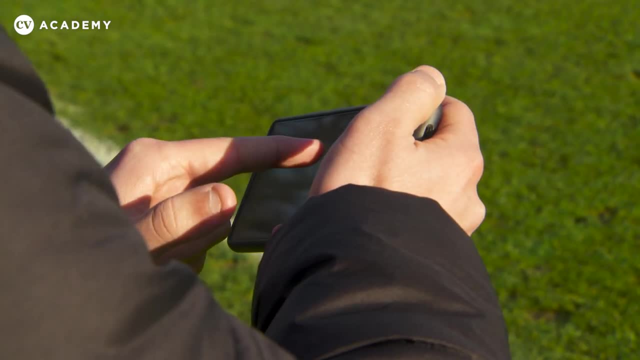 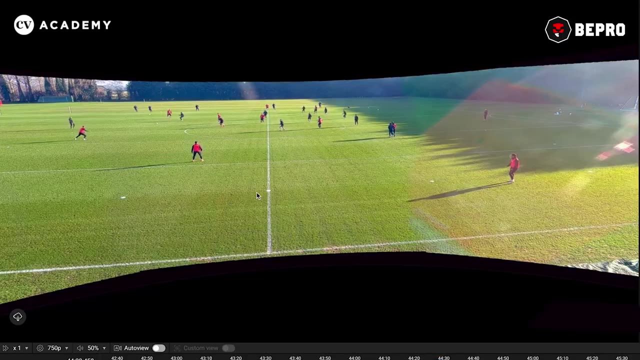 I could literally just get my phone up, see it go five seconds back. look at my phone, see the picture, confirm it, because at pitch level it's quite. you can sometimes think you've seen something and you haven't. 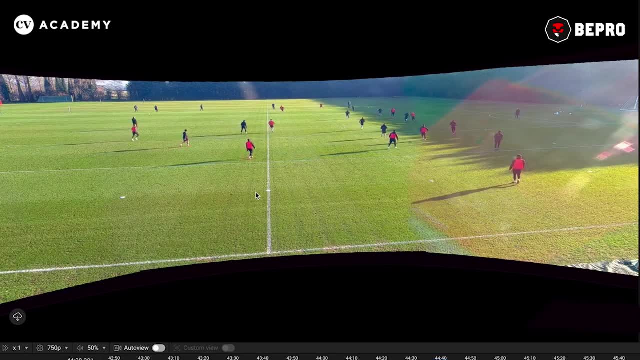 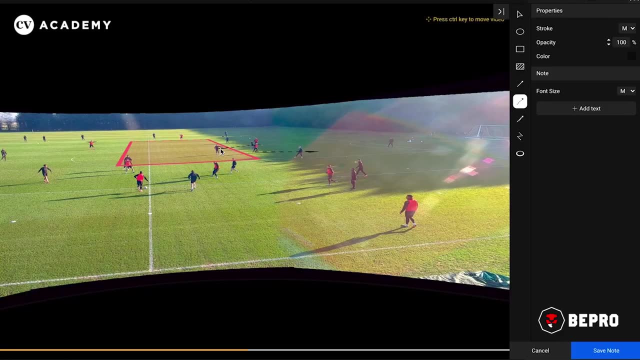 Confirm it, and there's just a little button you press. it's like a scissors button: You click on it and it just goes straight onto your library and your platform. So then after lunch I could just go back on that and see it. 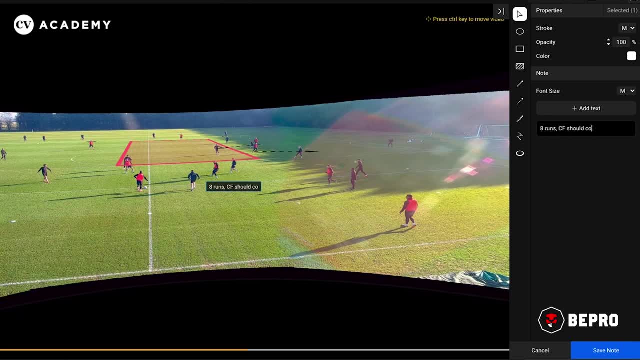 And then I'm going to in a bit, I'm going to push that one out to some players- probably the midfield and attacking unit, That's the thing that was missing in the past And that's the way it's where it's come a long way. 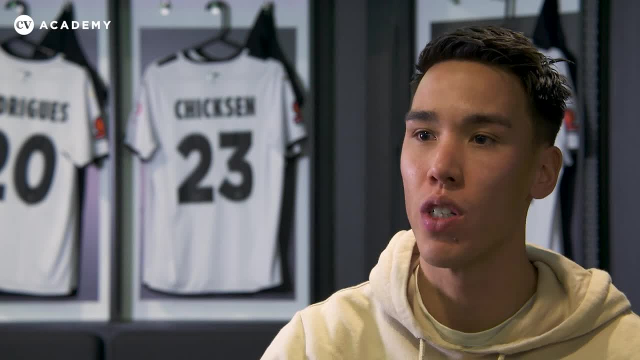 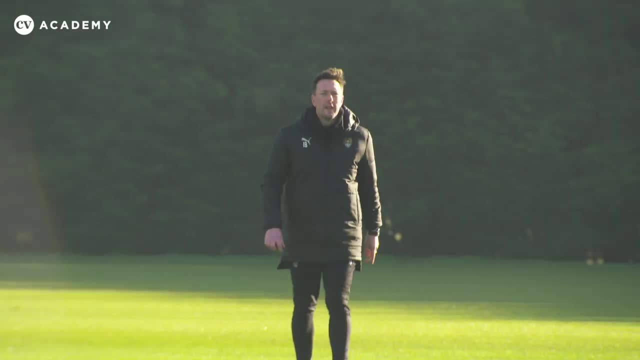 is because you'd have to do it visually on the training pitch. but then you're losing on on lads concentration to their load, to the. you stand out on the pitch agent and people switch off. here You can do it within instants. 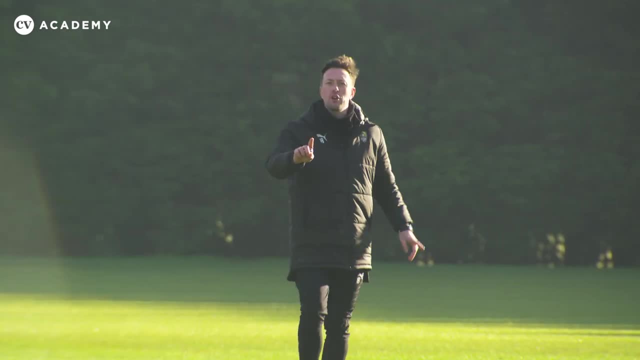 click it all done. done that within a few minutes you have the same point you have. then you would have going out and doing work in a whole- maybe two, three days to try and get across. You can get that within an instant of 15 minutes. 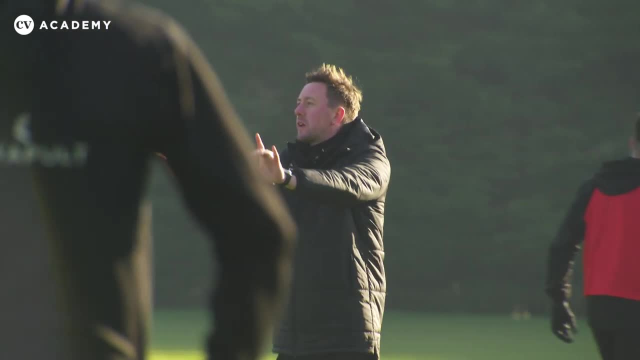 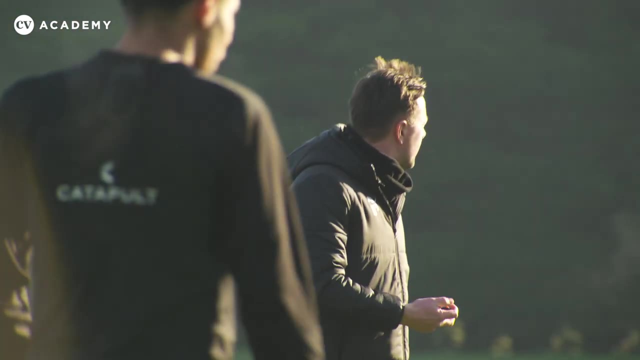 And I know for someone technical like the gaffer that's going to be massive because he needs to get his points across in a team view And and how he wants to play very quickly. We use it a lot for unit meetings as well. 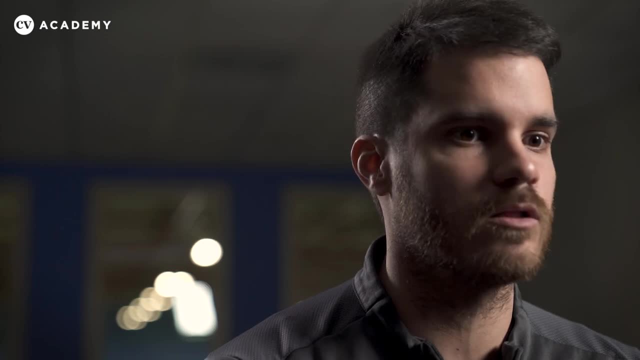 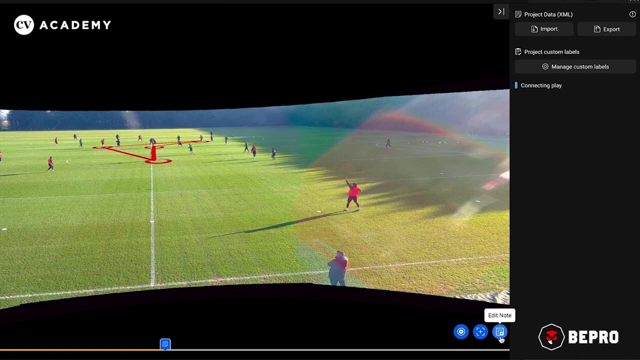 in terms of understanding what gives us success a lot and why things might've gone wrong. So we use it to see where the distances can get a bit big. So that's particularly important for for the defensive unit, but in general for everyone. 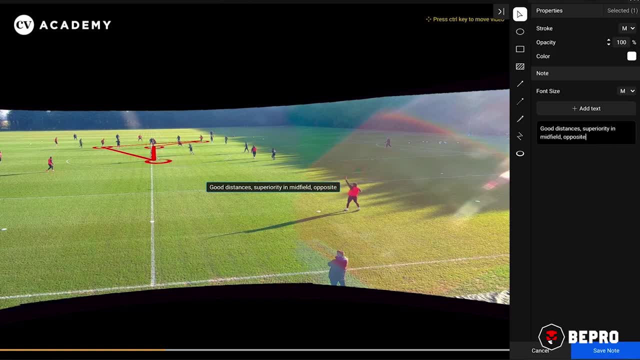 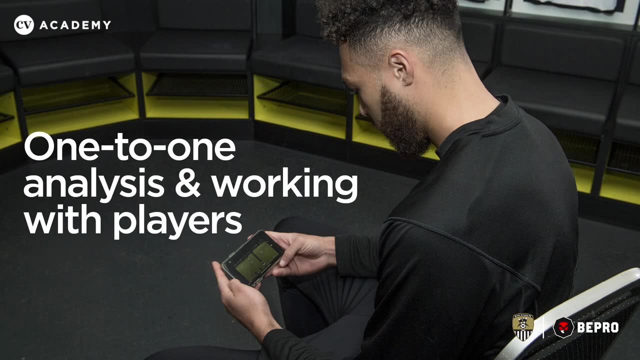 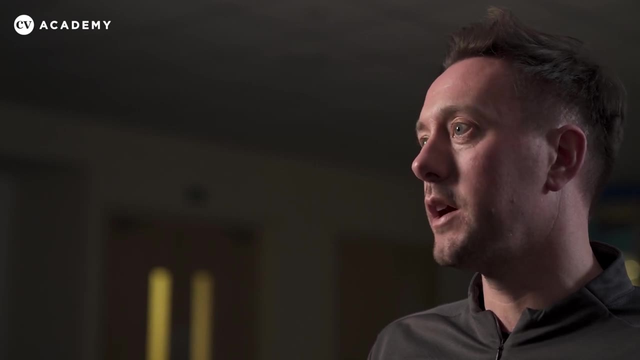 because that's. the other thing that we found is that a lot of it is everything's is linked. You need to create a culture within the group where the players want to be reflective and they're not afraid to look at the way in which they play. 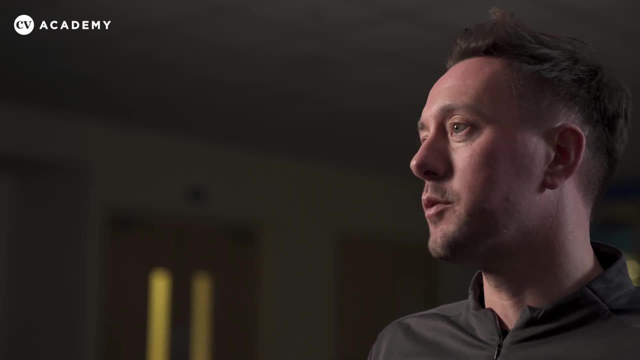 I think that's fundamental to analysis, that the players have to be open and not afraid to critique, And I think we try to create an environment where it's a discussion. You know, when we come in it's like we discuss the game. 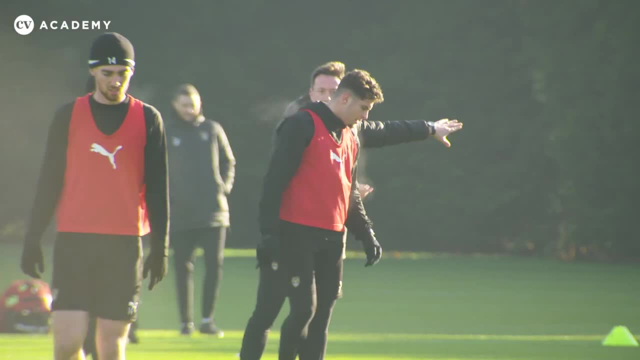 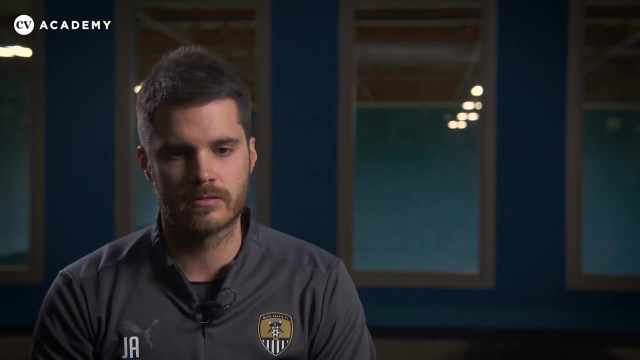 we discuss how we can improve and the players have to be on board with that. One of our centre forwards. we've basically used our training cameras to spot something that would have probably taken us a lot longer to spot if we didn't review our training process. 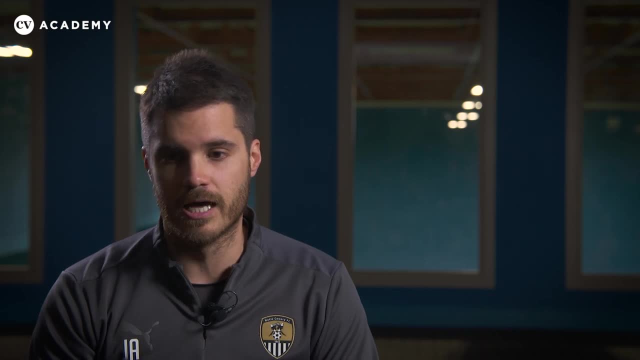 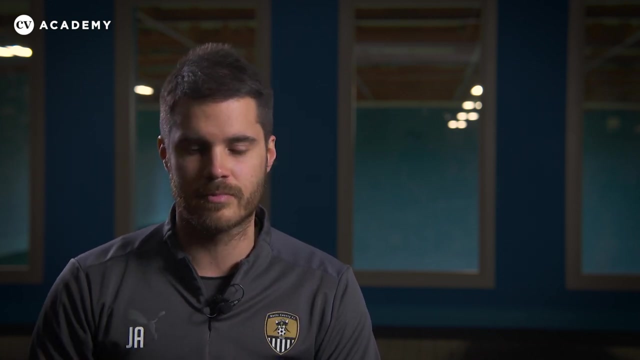 which can only happen with the cameras, with the footage, And we've realised that actually there was a little tweak in his movement inside the box that we thought would bring a lot of benefits to him, And after we spotted it it became a very easy. 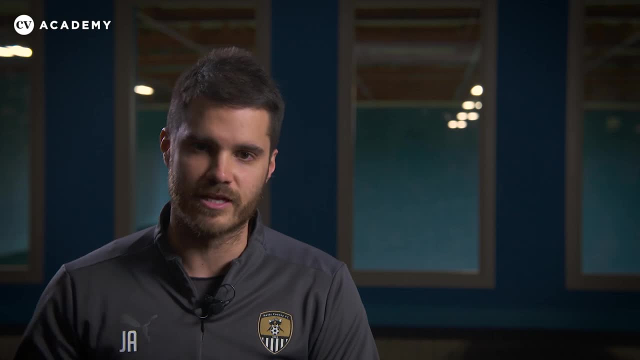 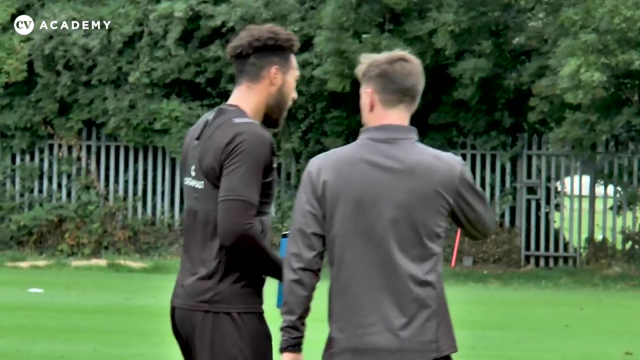 conversation to have, because we've then showed him the pictures and it became clear. and then we've showed him a couple of elite examples. I want to show you something afterwards. I watched the training back yesterday and looked at a couple of your movements in the box and I think it's something that we're going to work. 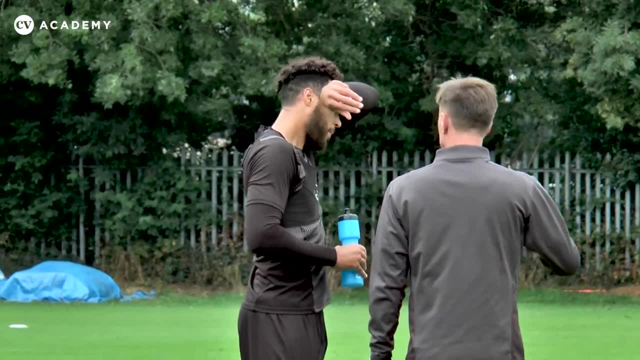 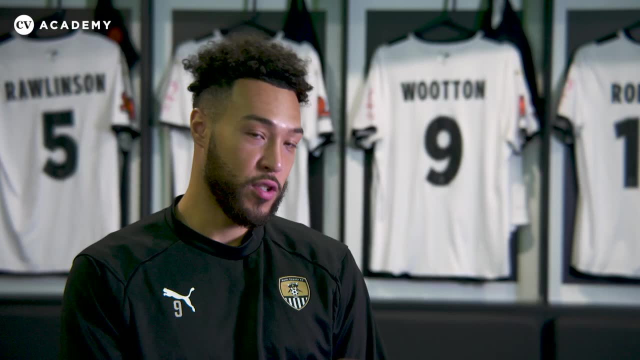 with on. I'm going to clip it today so we can go through it on Friday with some little things that I think will give you an edge inside the box. The manager said to me and we've watched certain clips of certain players. One was Patrick Bamford. 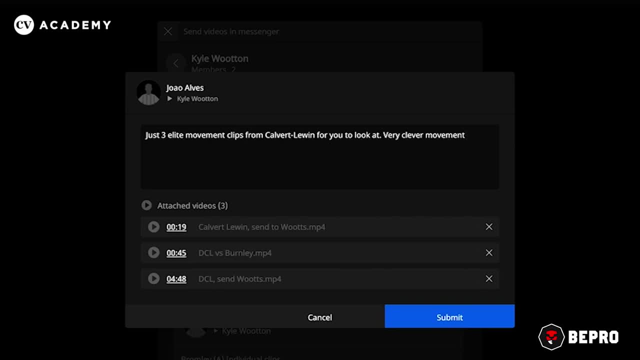 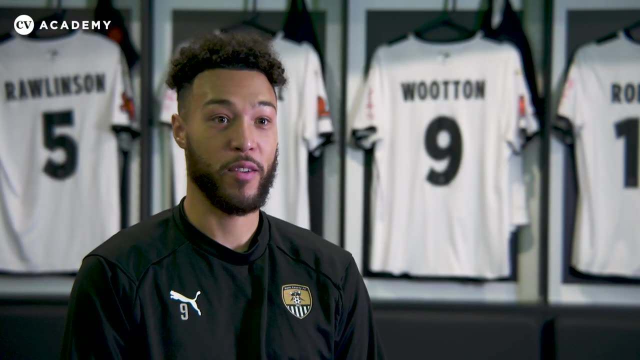 who we watched, and it was sort of the movement from taking the defender away to then attack the space, And it's paid off for me. I probably scored about maybe two or three goals from that, or maybe four this season. Ultimately, they're the people that are going to go on the pitch and play the 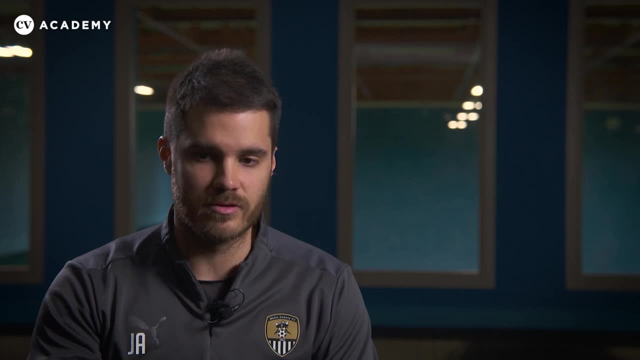 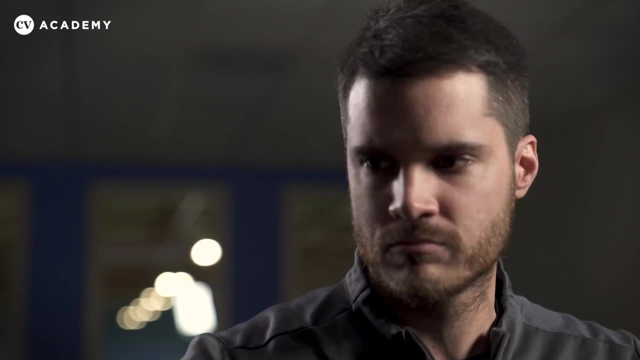 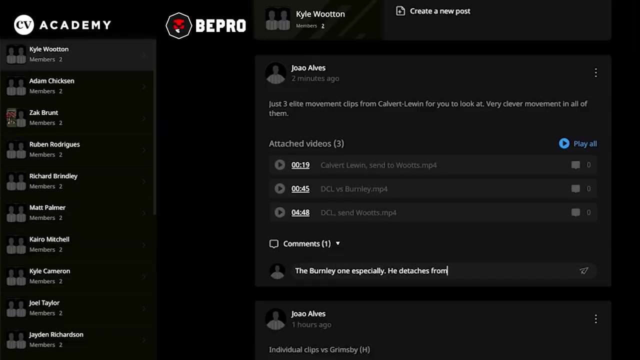 game and win his football matches, And so they're the important ones. So it wouldn't make sense to have a workflow where we can get to a million conclusions but then we can't actually pass it on to the players, And it's very important for us that the players can just open. 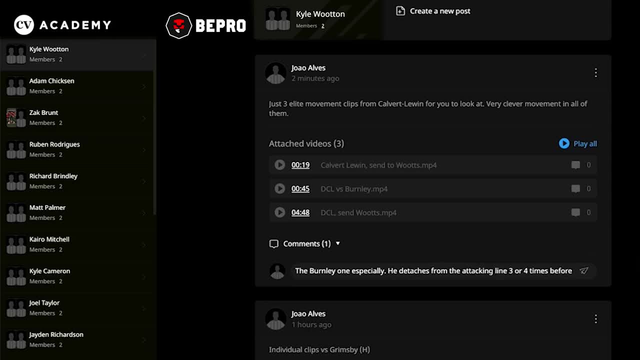 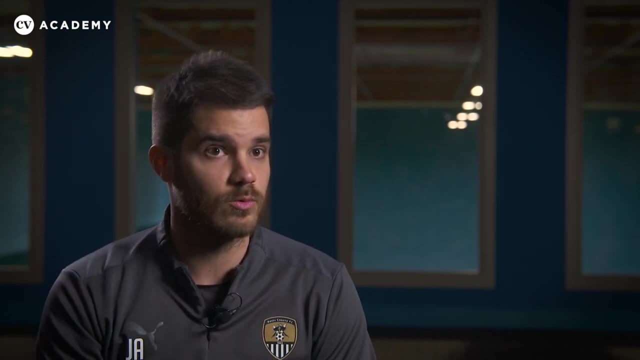 their phone and just quickly go on the app and they can go to their groups and open their individual clips or their unit meeting clips or the group ones, the big ones. They can throw comments in to ask me or ask the gaffer or ask whoever it might be, what they think. 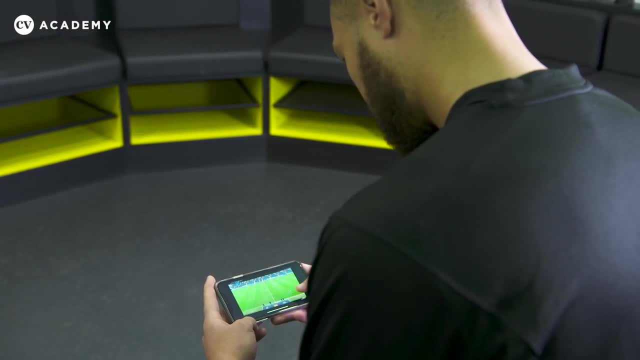 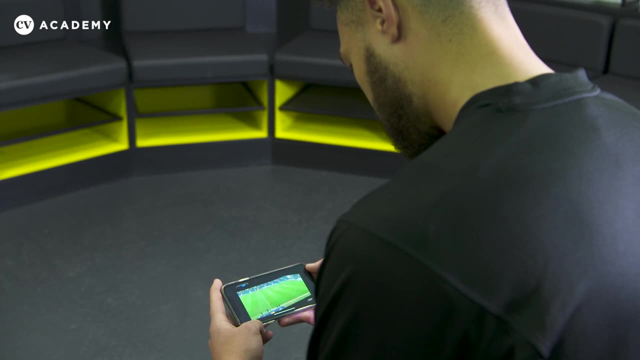 Xiao sort of got that across when we first started using the Beepro app, But as it's gone on, everyone's interacted. moreover, Yeah, I mean the coaches have got really involved in it as well, which I think is good. 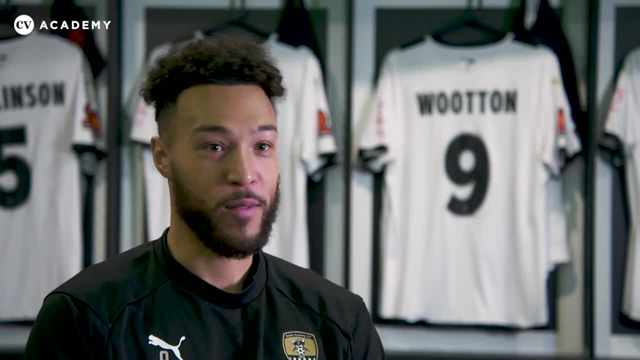 Now I speak to Sam Slocum, the goalkeeper, and every morning we have a conversation about: oh, did you see that back, Or did you see this, what we could do better? Pretty much after every game there's always something. 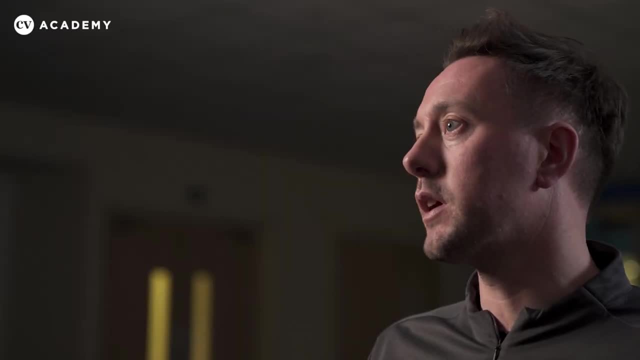 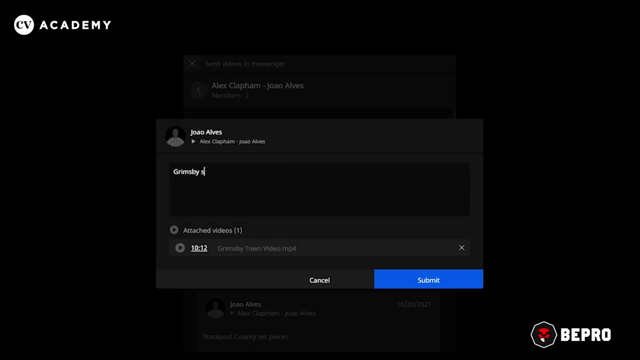 I mean we tend to upload the games onto the Beepro system and then we can clip it down. I think it's been very good for the set plays, where we can have specific set play groups and then put in some of the opposition set plays into that so that the players can access that through the 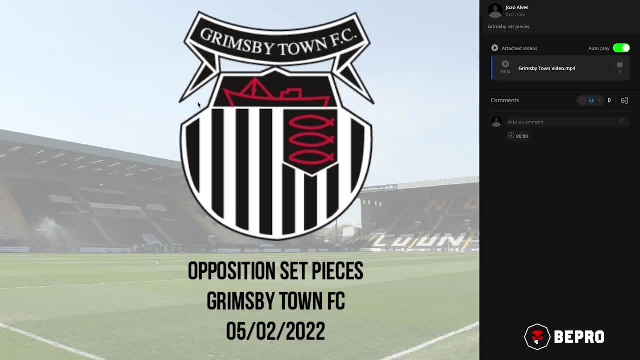 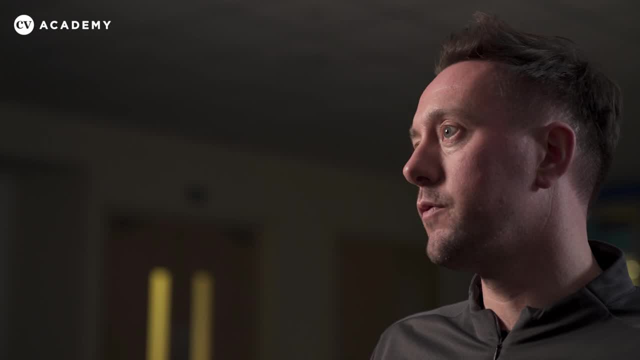 week And we tend to have a main full team meeting around opposition analysis, But then following that we can put more specific clips onto the Beepro for the. so if we have a defending group we can put the opposition attackers on their common movements and 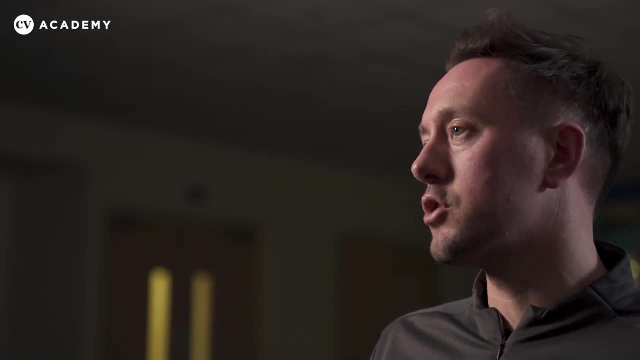 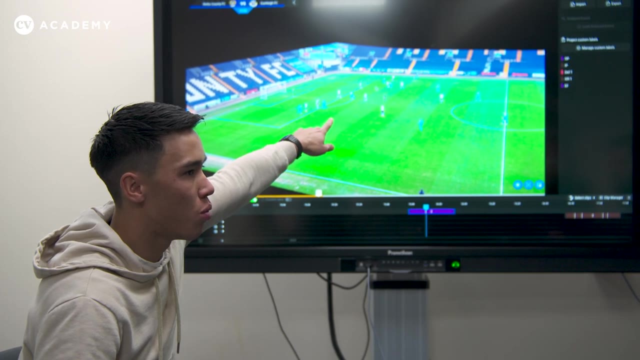 trends. So I think it allows us to break it down and chunk it to the players and give it to them that way, Because, as it goes out there, Yeah, stay in your slot. It's a right back. It's only going to stand on the ball and pass back inside. 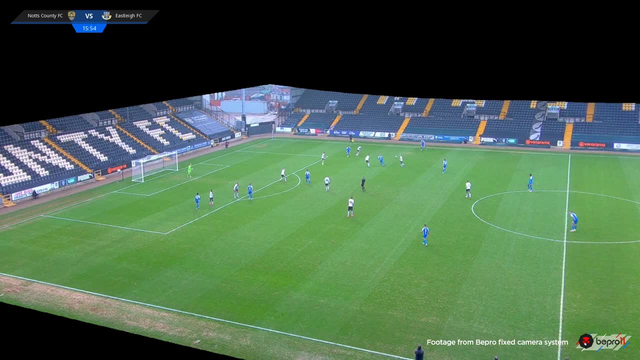 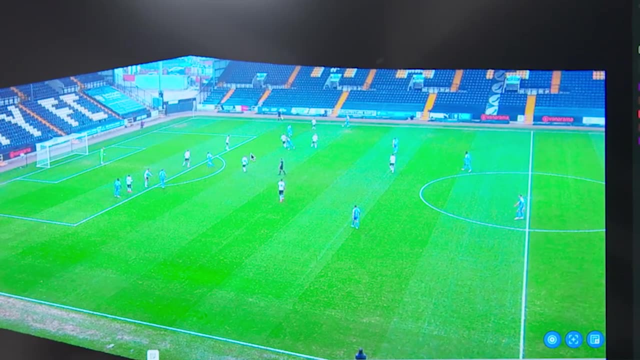 He's more dangerous. That guy's more dangerous there. That guy there get goalsigned. I've heard of him. Of course he's more dangerous. He's more dangerous as it goes wide out and then, as he goes further down, come out. 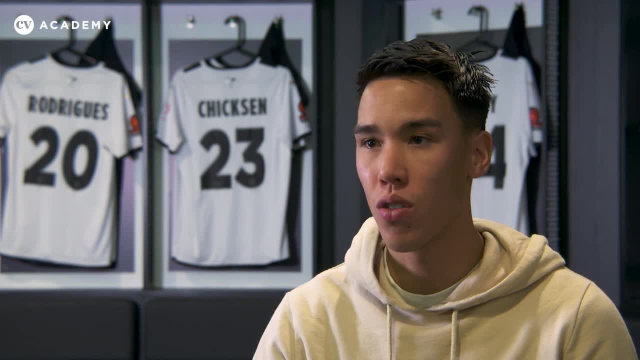 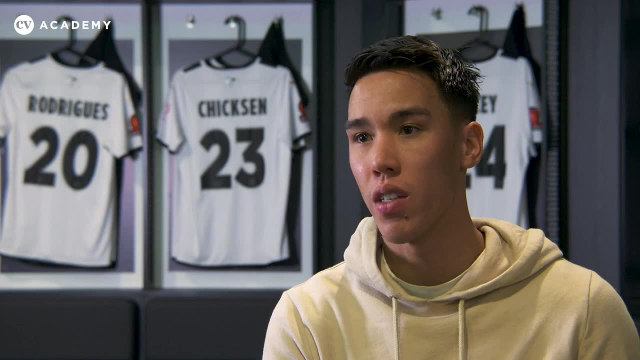 For me. I like to clear my mind, before I get there, of what the good and the bad traits of a winger is. Once I know that, or even if it's a defender, once I know that, I put it to rest. it's in my mind. 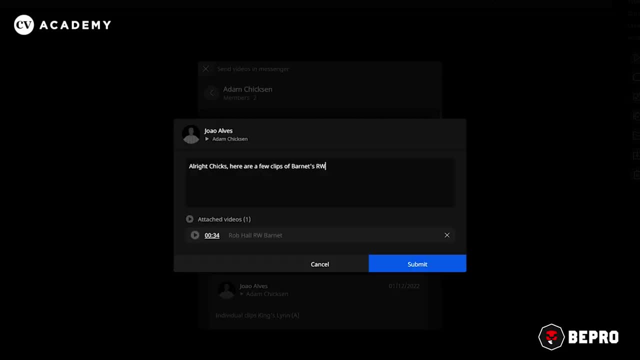 it's to rest. So then my whole thought shifts to how is he going to now worry about me? So I analyze quickly as possible, know what I'm going to be dealing against going through with you And that's it Me. I like to do it earlier. 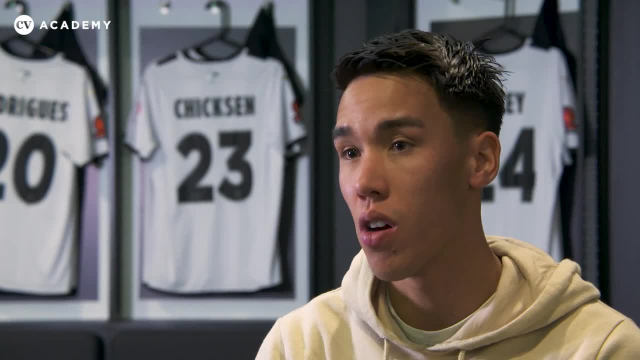 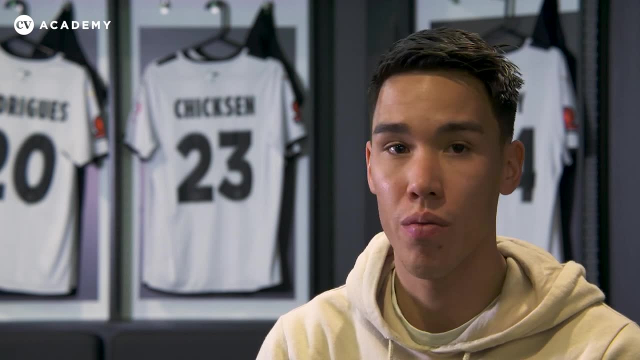 maybe on a lighter day, because I find if you're doing it after a hard session, can you take in and process the amount of information that the B pro. it's like anything if you get nine to five job and you go all the way to the end. 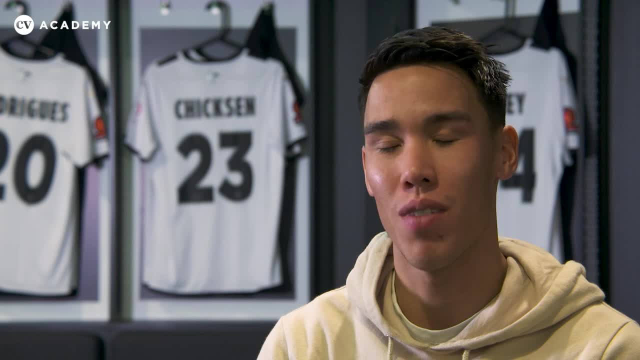 of the day and you say: right now we're going to analyze your day and what I mean. you just want a cup of tea and you want to sit down next to your wife and just relax for a bit here. It's the same thing. 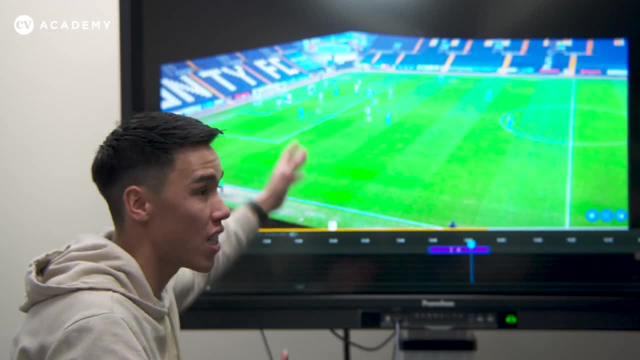 I want to do it where it's going to stay and stay sunk in. He's that tight in the box. It only takes that. that, Yeah, And then he gone. That guy nearly just scores. You know what I mean. 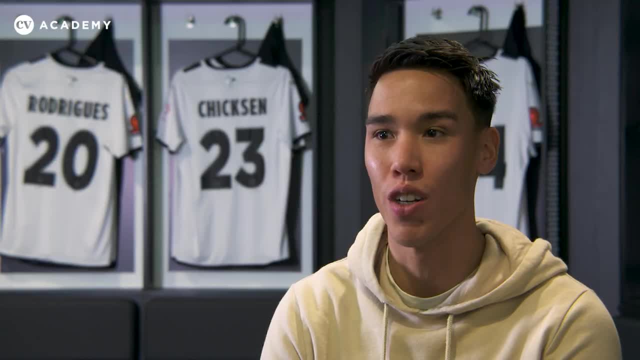 Yeah, definitely Old I've got. you see the same things. but you just want to know that you're seeing the same things because- and that's why analysis is so important- because if you come too safe with it and say, Oh, 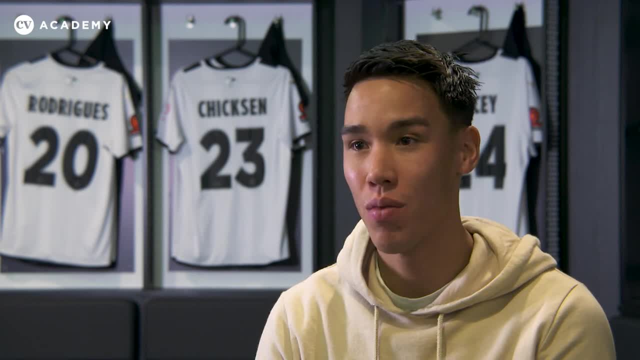 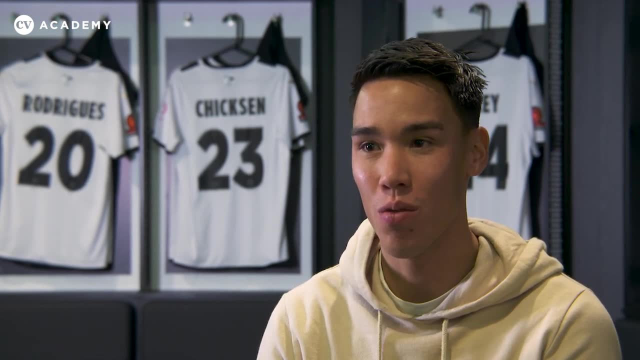 you think you know there'll be a guy that does something completely out of different or new or something random that you don't analyze, and then you're getting left behind again or you're having you're dropping the team's performance because you haven't looked into it. 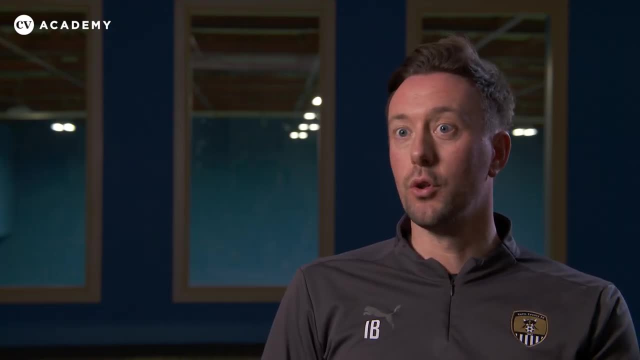 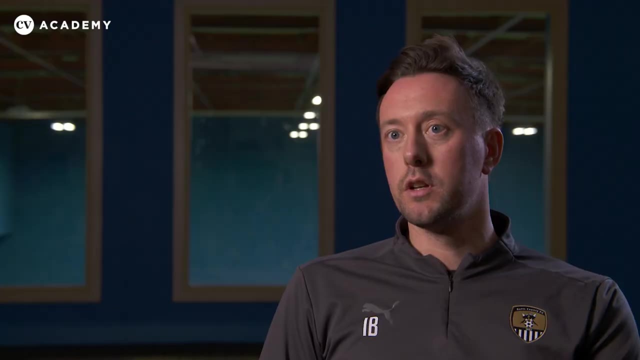 You want to have things that that push your work, So we want to have more things to work on. So normally the more advanced you get with the technology, the more access to stuff you have, but certainly it makes us more efficient in terms of if you take an. 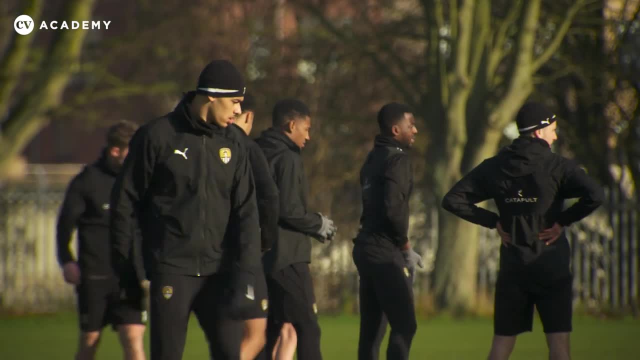 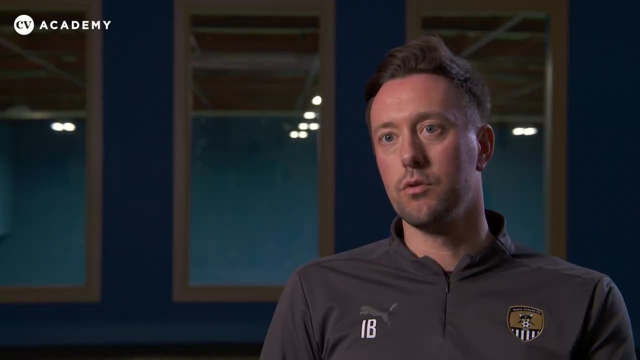 overall season and the ability to get all of your messages across and how you want to play. the more information you can get to the players in a short space of time means that you're more efficient with that. It allows us to give stronger, clearer feedback to the players quicker, to make our overall 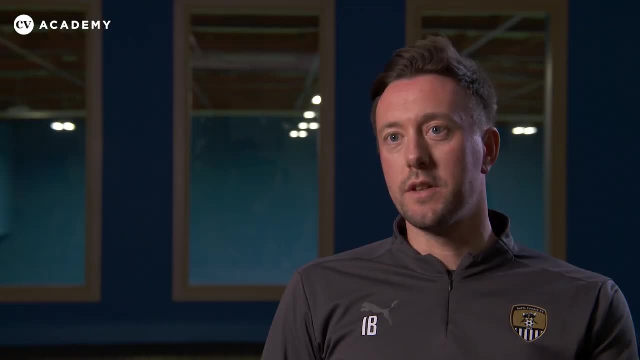 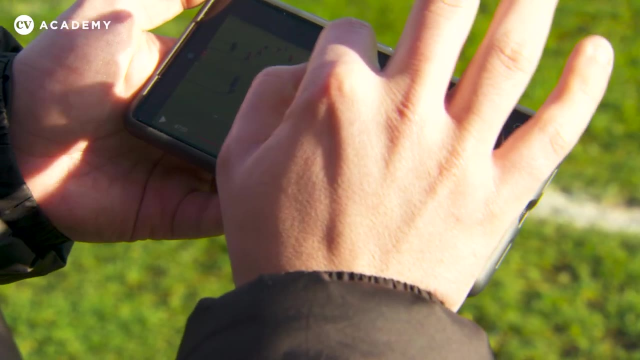 process of developing the team much more efficient. Almost everybody spends a lot of time looking at their smartphones, So I guess, to be able to have access to all the things that you need and the information around, an upcoming game at your fingertips on your smartphone is. 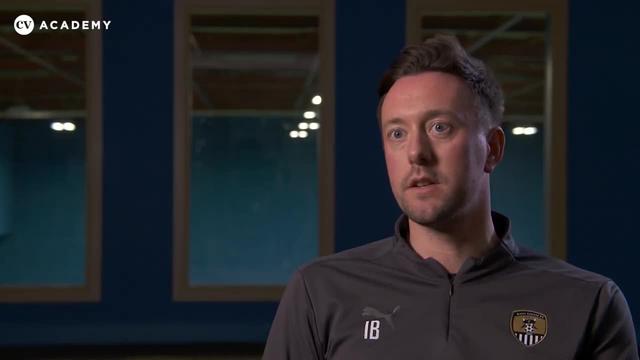 is a huge benefit really, so that it's so accessible for the players. There's no excuse really for for not being aware of opposition or your own strengths and weaknesses or your own reflections on the last game. So I think it gives that accessibility and it stops players only being 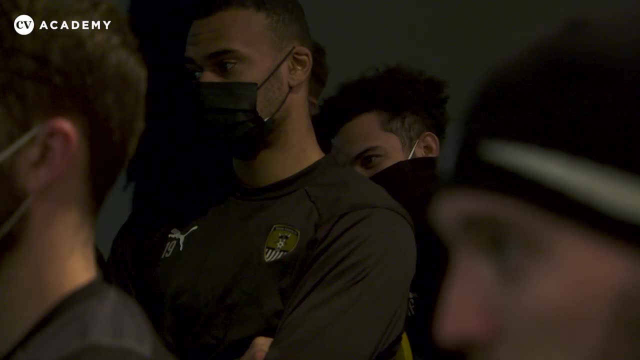 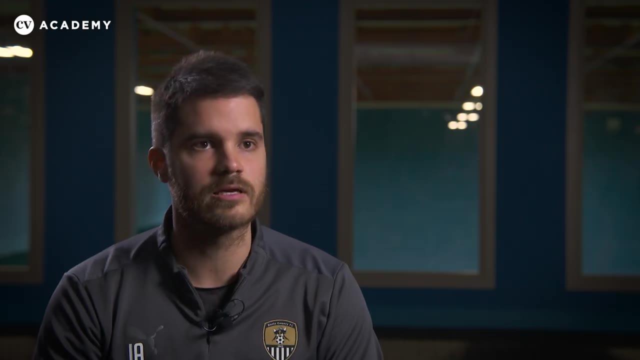 spoonfed, waiting for a big group video analysis or one-to-one. They can take some of the initiative on the analysis themselves and have opinions on it, which is great. It becomes very clear when you've got pictures, basically, and if the players can see them. 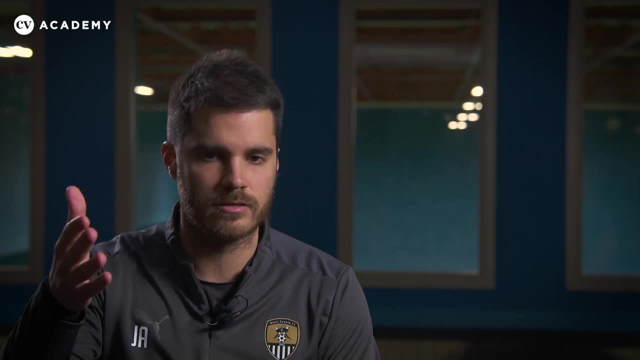 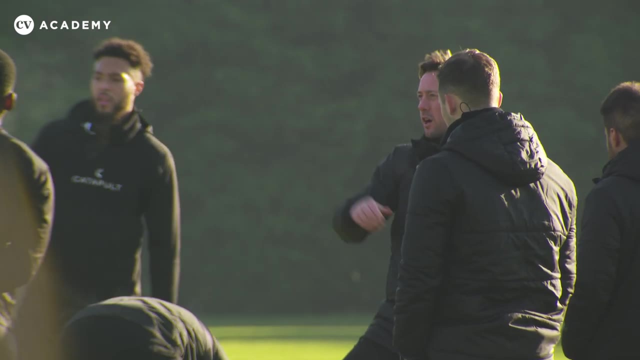 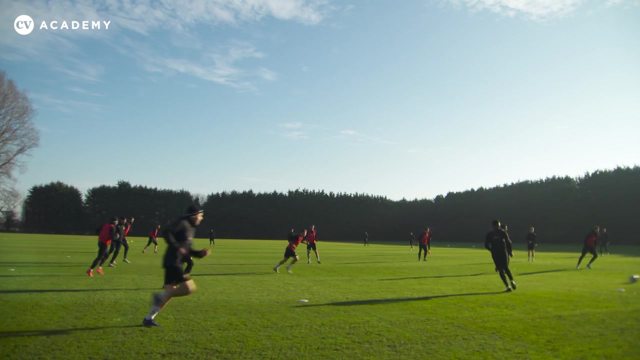 you can. you can be a lot more certain that they understand exactly what you're trying to put across. The B-Pro cameras: they're very important to us in the sense that they help us get the pictures, have a nice platform where you can just store stuff and share stuff with the players as well. 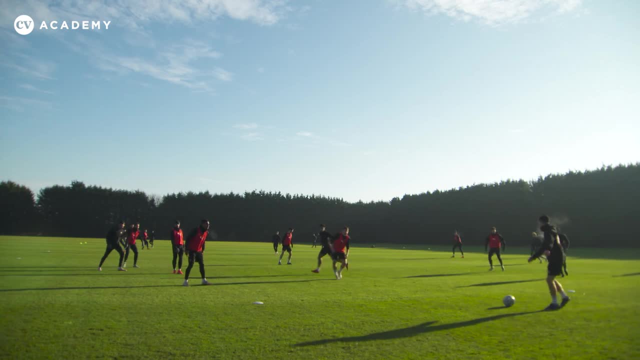 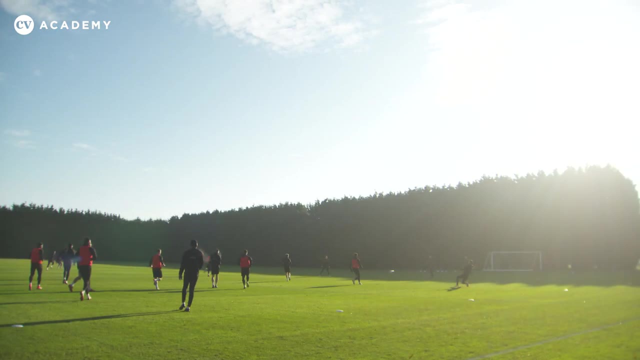 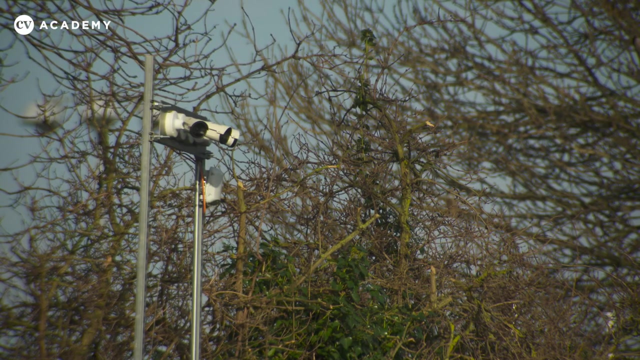 So it all just filters into that one platform, rather than me having it on different folders on my laptop external USB drives. I don't actually have to man the camera, So they've installed the cameras there. with the training ground, One's got decent vantage. 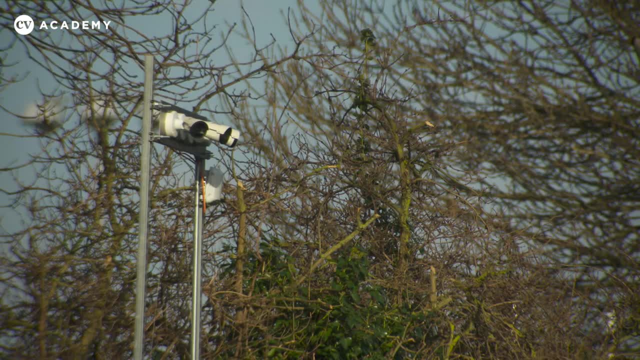 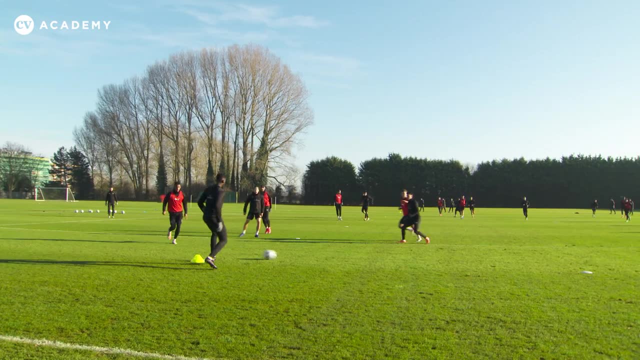 the stadium, definitely really good vantage as well. So that's one of the struggles I used to have before B-Pro was to see the stuff that I needed to see. while operating the camera It became very clear that it's I was either going to do one or the other. well. 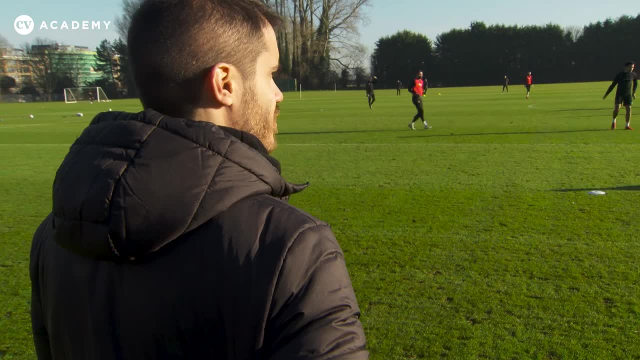 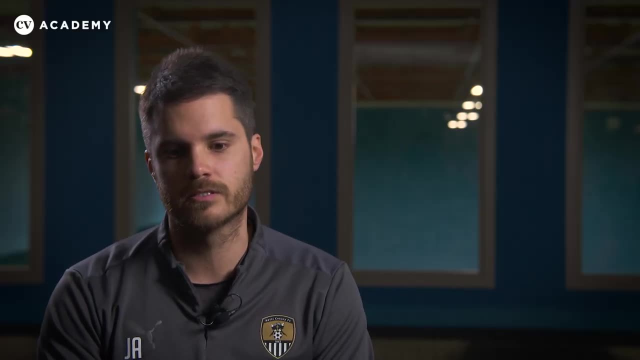 I ended up panellising- better than filming, if I'm honest, So that's saving me a lot of hours- The storage, the organisation, all of these little things- I think it's from my perspective, anyway, because we do pre-match. 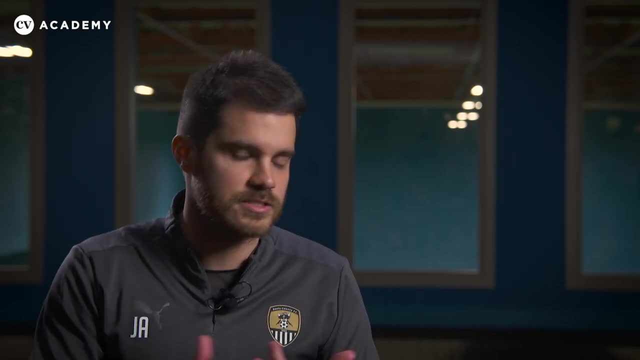 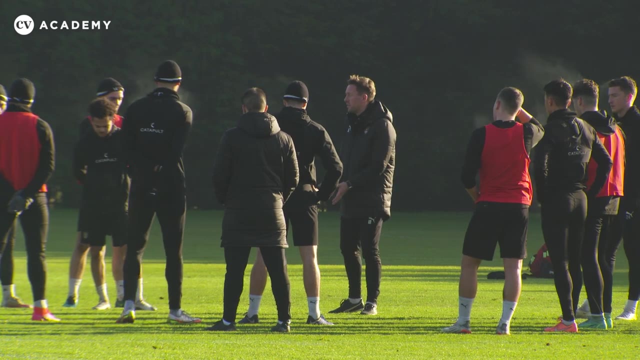 post-match training: individual bits. it's very easy to get disorganised And to have clips here and there and everywhere or not rename one, or right now I know that all my clips are there and that's helpful for me for sure. 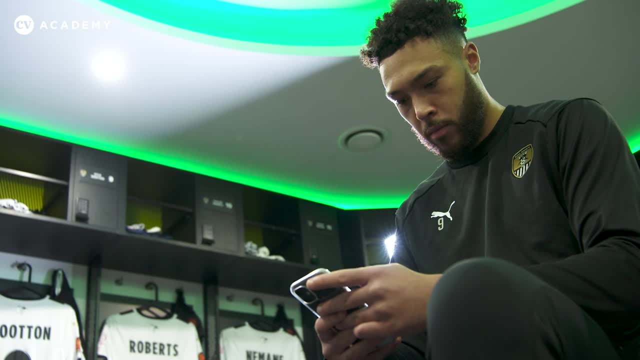 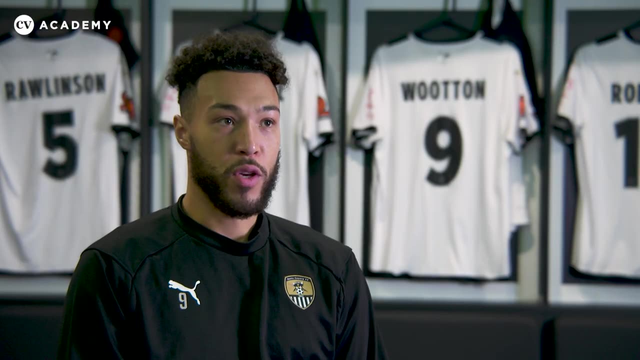 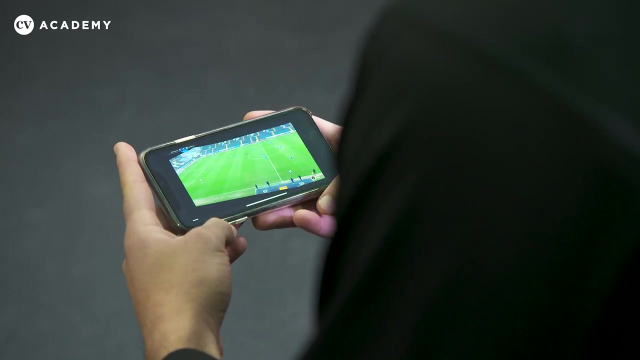 And it definitely makes me more efficient. Yeah, When you can see it and you can watch it over again, it's a massive help for me. anyway, We can literally watch it whenever. Usually, we receive the video of our individual clips from maybe the next morning from a game. 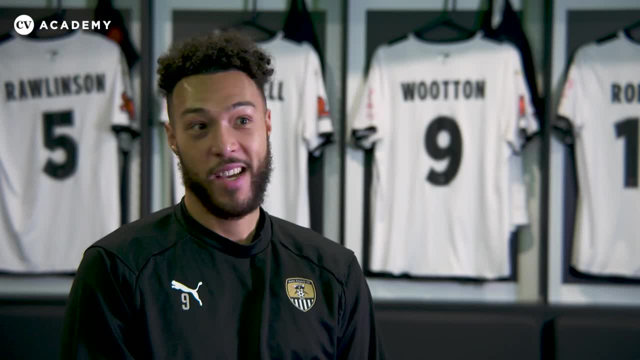 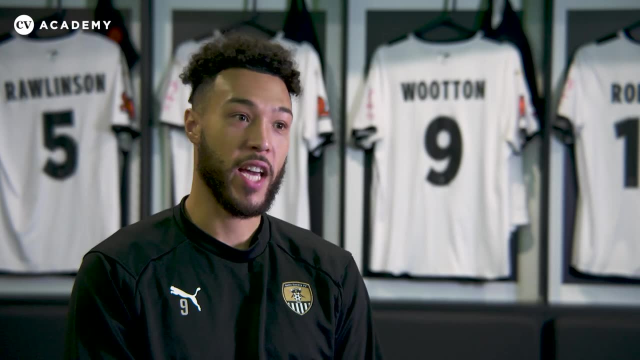 So I just literally go through the whole of my clips. it might be it could be 40 minutes, could be half an hour, but I think it will always help you for any player If you want to get there and you want to be the best you can every day and be the best for the team. 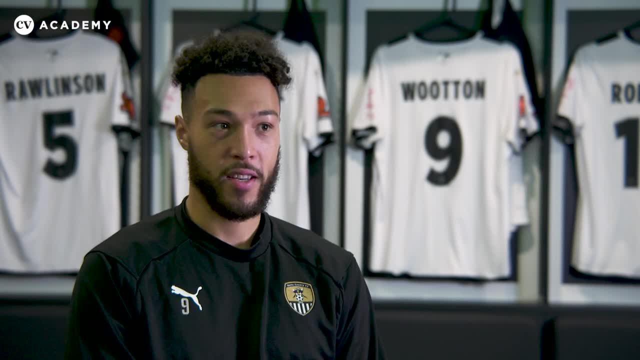 then it's going to be a massive help. I mean, you can watch things and take things on board. Even in the training session today I spoke with Xiao and he said: oh, one thing, one movement, here you can do this. 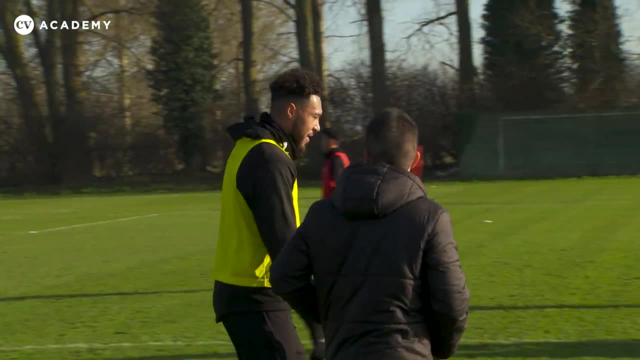 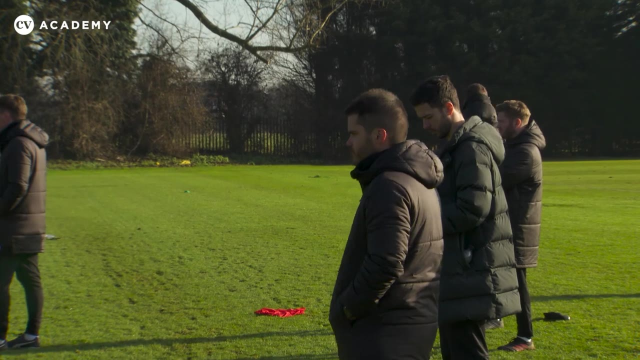 You can stay away and peel because he can then pick if you want to go left or right. Do you know what I mean? Yeah, Especially for our level at National League as well, I can't imagine many teams having the same spec and high spec of analysis. 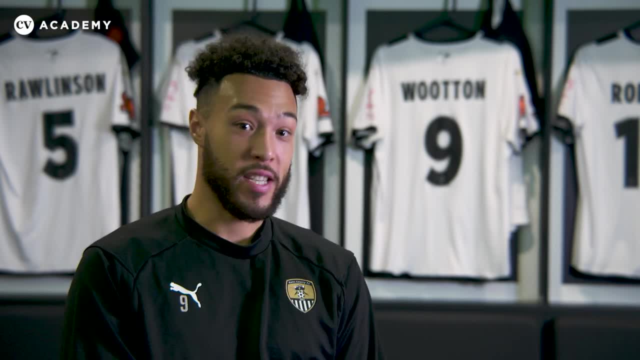 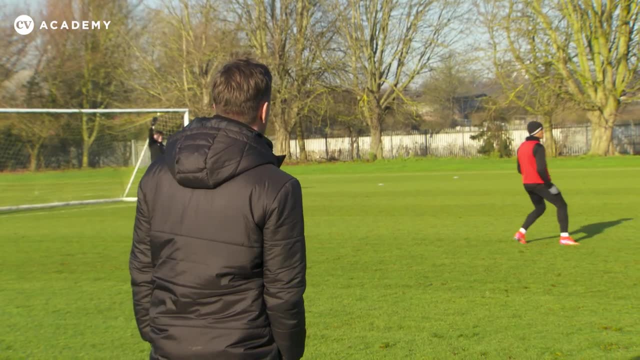 So no, like I say it's huge for us and I think throughout the season it's only got better and I think the lads have took on board. literally week by week It's improving and you can see it out on the pitch. 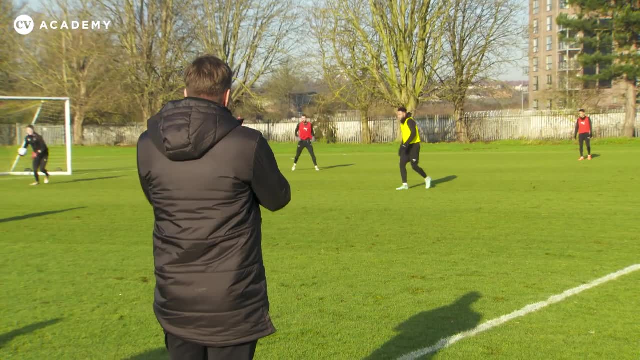 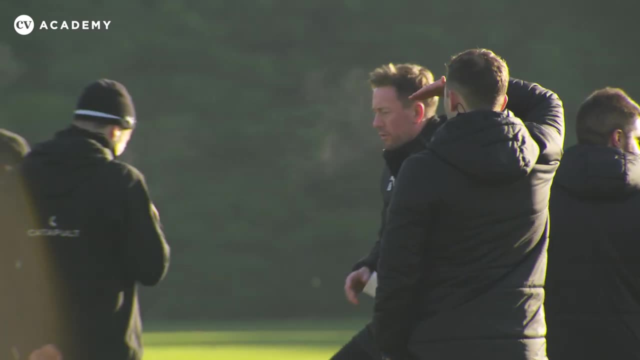 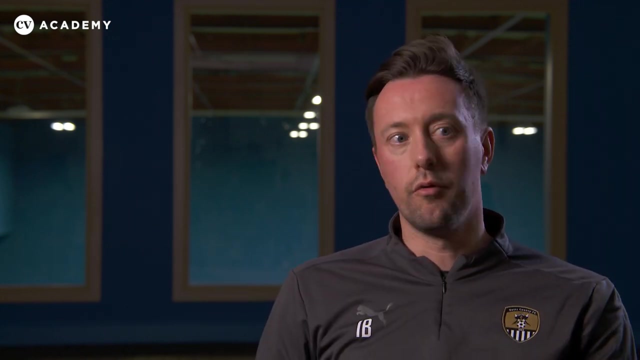 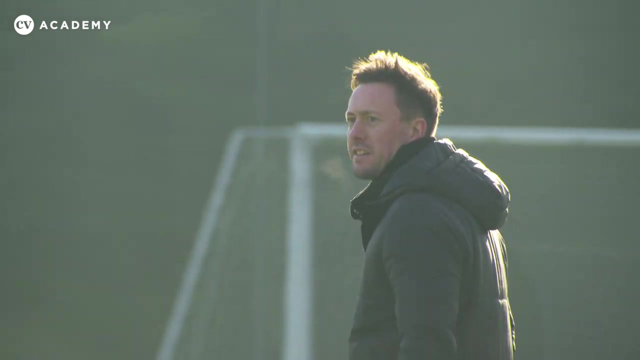 The evolution now has meant that there's more accessible and affordable quality analysis and the knowledge and input filters down. So, as it gets even better, at the very end, at the very top, it filters down. So now we're coming to National League and I know there's a lot of teams in this league that are very resourceful in terms of analysis and it's evolving a lot and that's only good for the game. 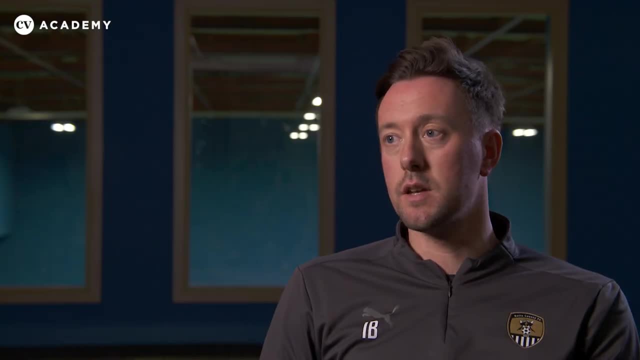 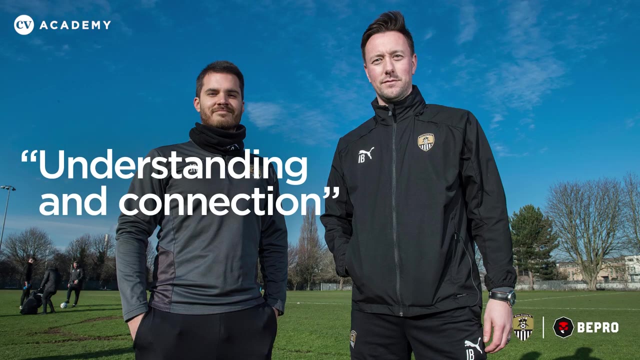 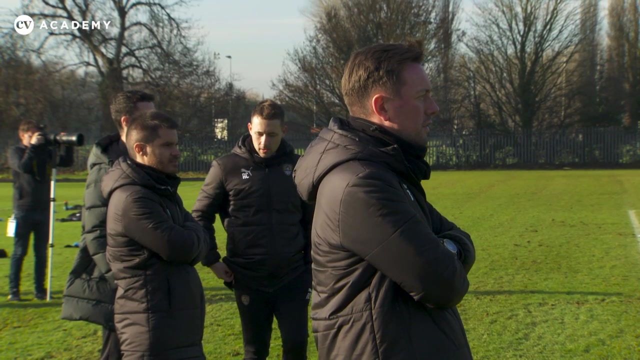 for the development of the players in the league, that teams further down the pyramid are able to access really good resources around analysis. The more you work together with staff- I think not only analysts but physical staff and medical staff- I think everybody starts to understand how you want the training and you start to connect there. 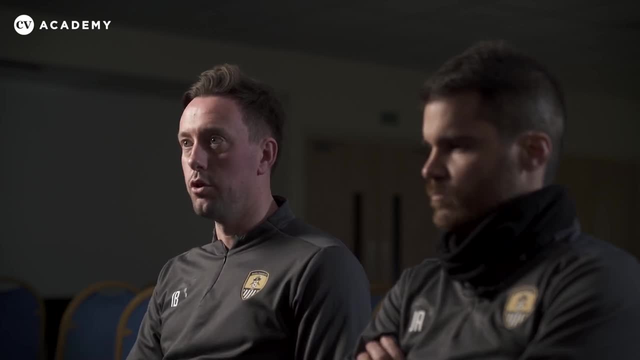 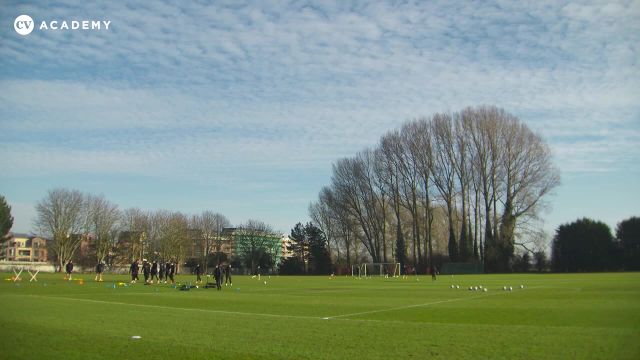 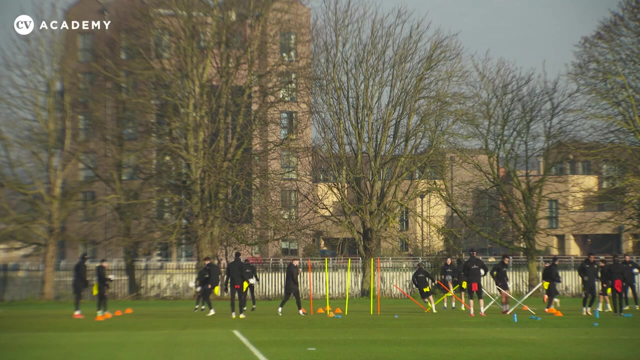 So, obviously, that you become very close, close knit group and understanding each other, each other's roles and certainly how we want the final picture to look, is massive, I agree. I think it's such a big operation in running a football club that we need to have this understanding and connection, and he puts you at ease.